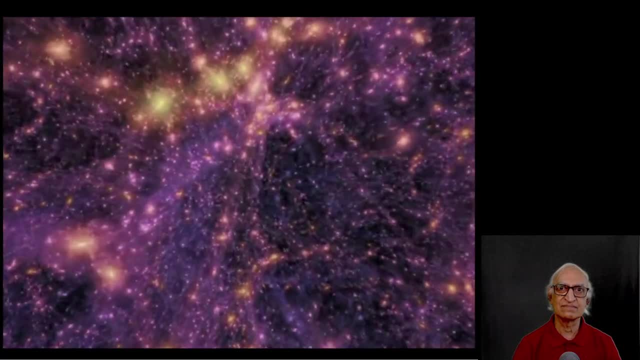 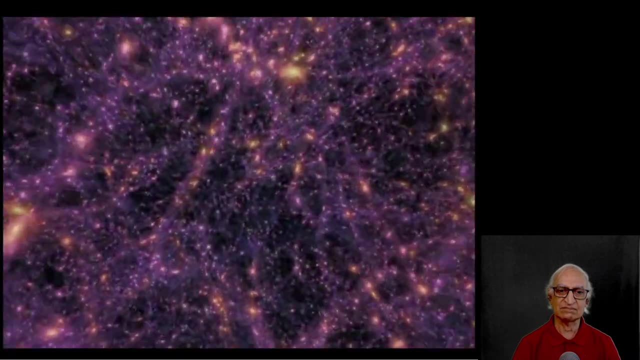 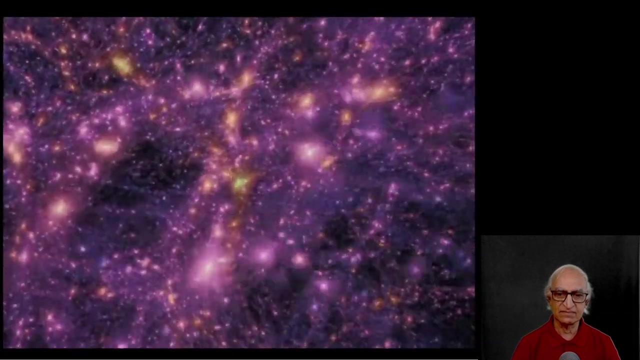 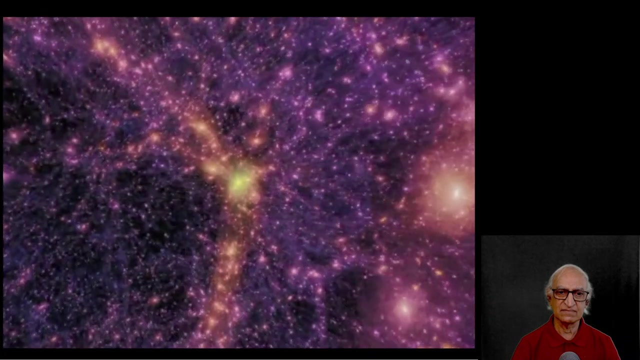 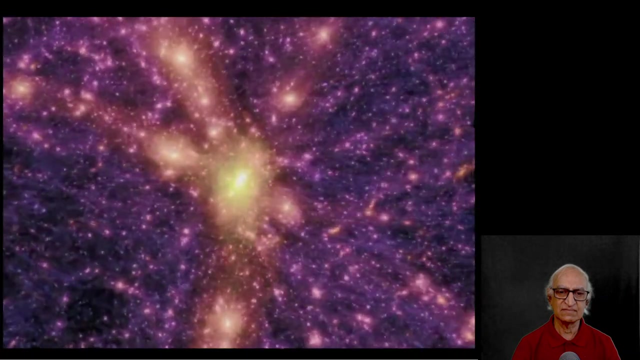 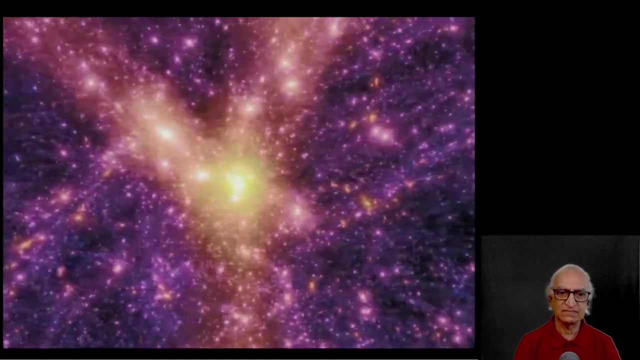 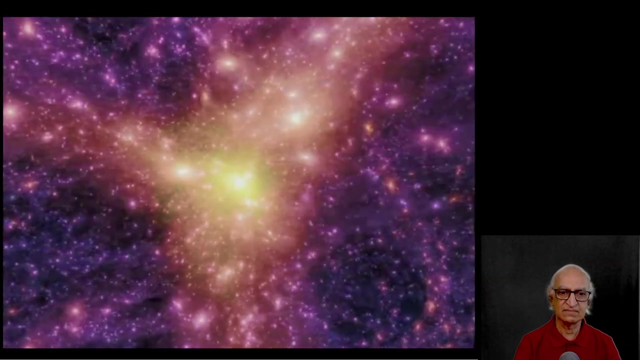 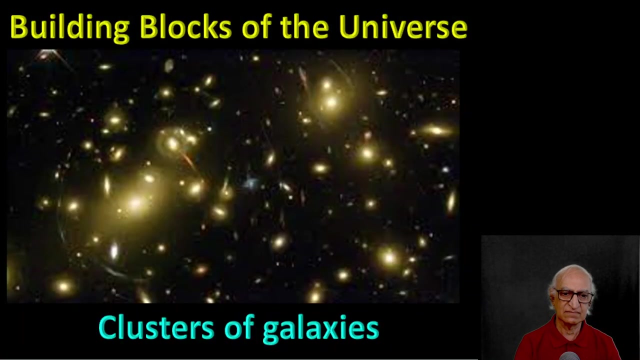 Come with me. The building blocks of our universe are clusters of galaxies such as the one you see here. A typical cluster of galaxies will contain several hundred to thousands of galaxies bound together by mutual gravity. There are billions and billions of such clusters of galaxies in our universe. 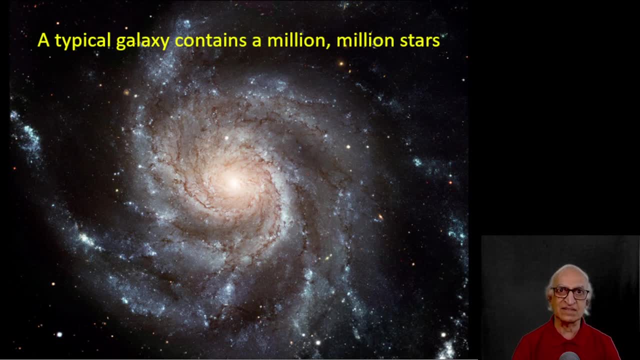 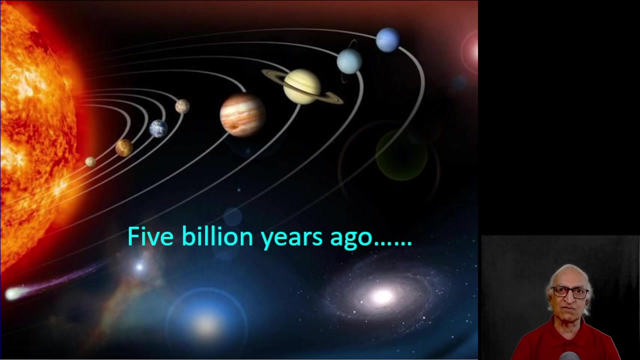 The building blocks of the clusters are individual galaxies, such as the one that you see. Each galaxy typically contains a billion million stars. In one of those 350 or so billion galaxies in the universe, some five billion years ago, a star was born with a system of planets revolving around it. 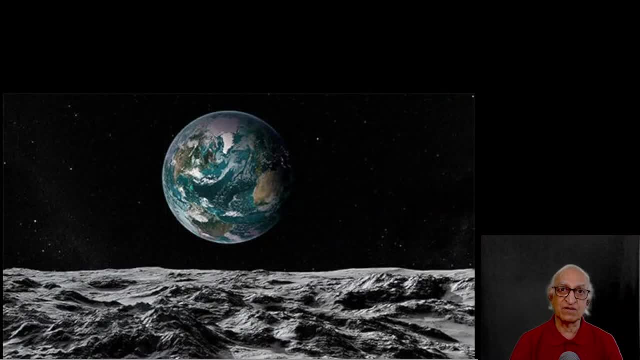 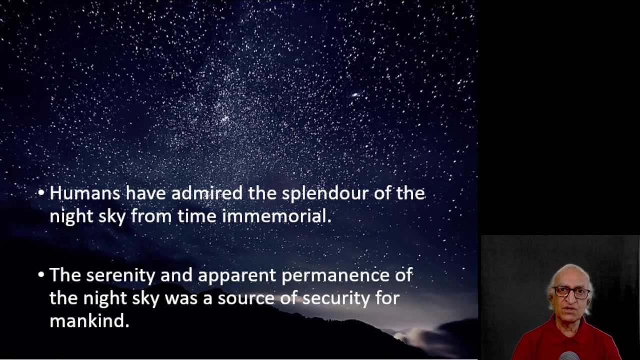 In one of those planets. roughly four billion years ago, life forms first originated and evolved to more complex organisms Roughly 300,000 to 200,000 years ago. thousand years ago, sapiens first appeared on this planet. Humans have always admired the splendor of the night sky from time immemorial. 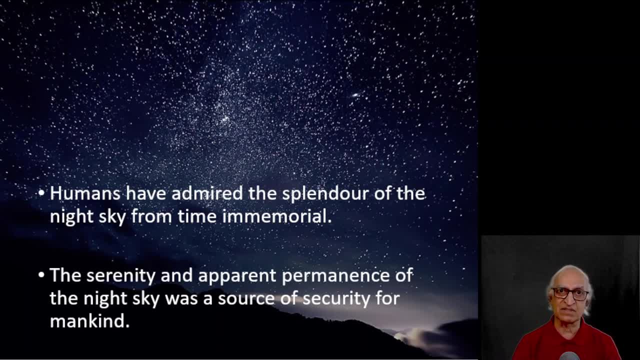 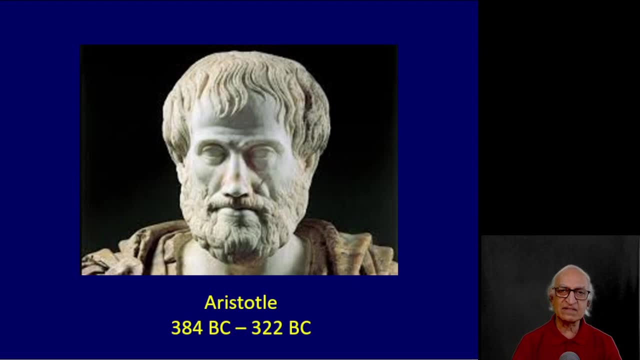 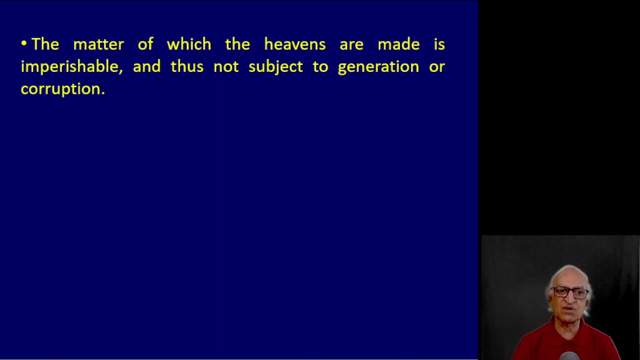 Indeed, the serenity and apparent permanence of the night sky was a source of security for mankind. The great Greek philosopher, Aristotle, enshrined this into the philosophy of the universe. According to Aristotle, the matter of which the Heavens are made, 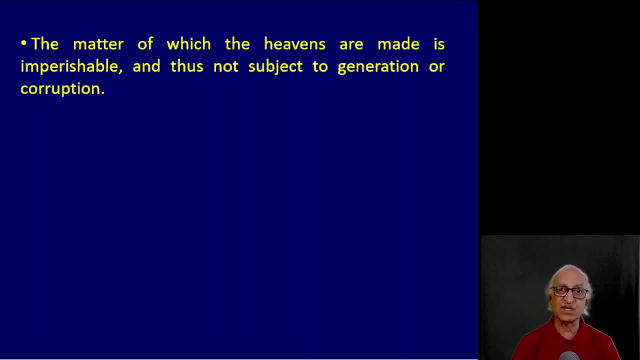 is imperishable and thus not subject to generation or corruption. In contrast, the earth is made up of the classical elements earth, water and means air, fire and is perishable. The motions in the heavens are eternal and perfect. The heavens. 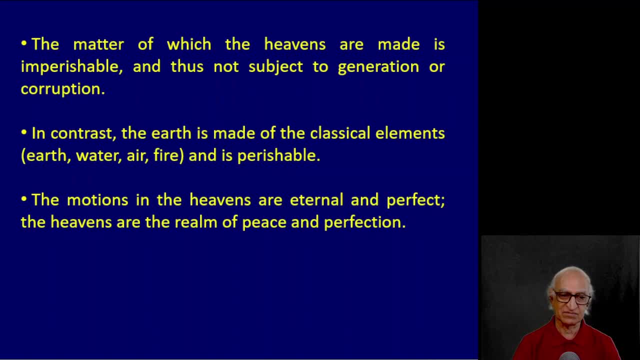 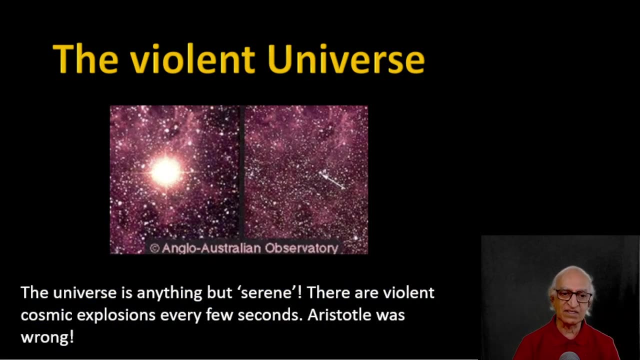 are the realm of peace and perfection. This was the Aristotelian view of the universe that dominated Western thinking for over 2000 years. Unfortunately, the universe is anything but serene. There are violent cosmic explosions every few seconds. These explosions are so violent that the energy released in a typical 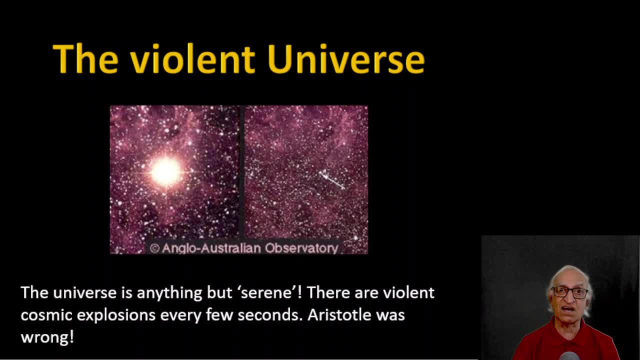 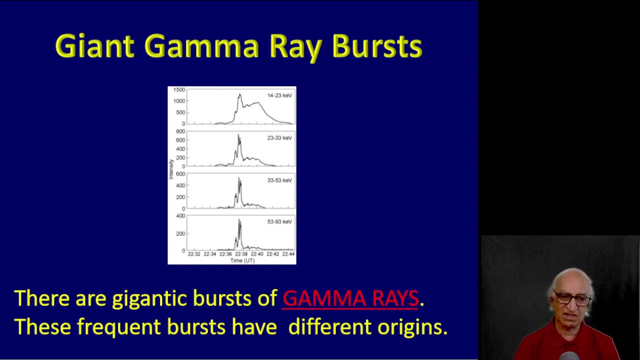 explosion far exceeds the energy a star would have radiated in its entire lifetime. So Aristotle was wrong. These are not the only explosions that we see. There are gigantic explosions. There are gigantic explosions. There are gigantic explosions. There are gigantic bursts of gamma rays. These frequent bursts have different kinds of origin. 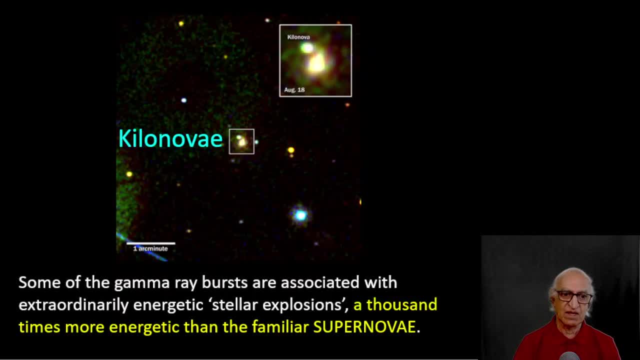 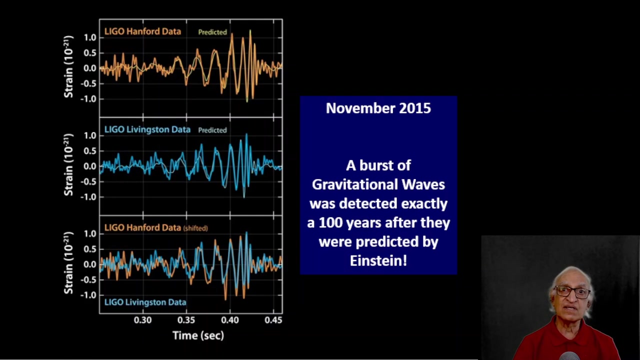 and we shall discuss that later on. Some of the gamma ray bursts, at least, are associated with extraordinarily energetic stellar explosions, known as kilonovae, a thousand times more energetic than the familiar supernova explosion of stars. And these are not the only finals. In November 2015,, a burst of gravestation. 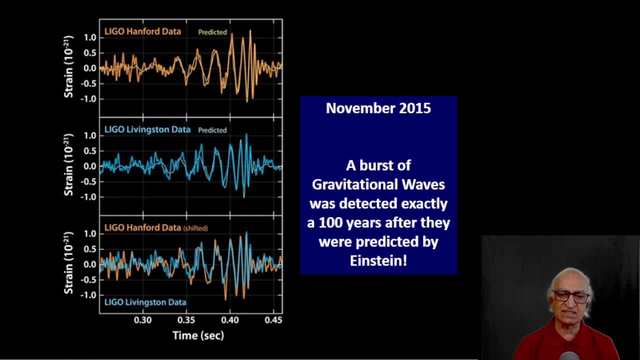 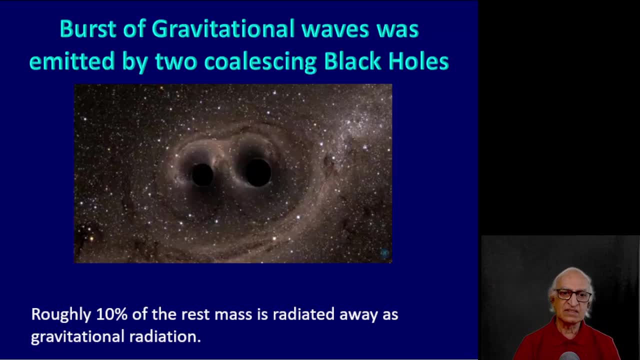 of waves was detected by Einstein's General Theory of Relativity exactly 100 years after the expected effect experienced by Einstein's Johnา knot in Einstein's general gradient argument. geological influence- Sie. geological influence, Sieérica. geological joka. This burst of gravitational waves was due to two black holes. spiraling inprints, C Trade. 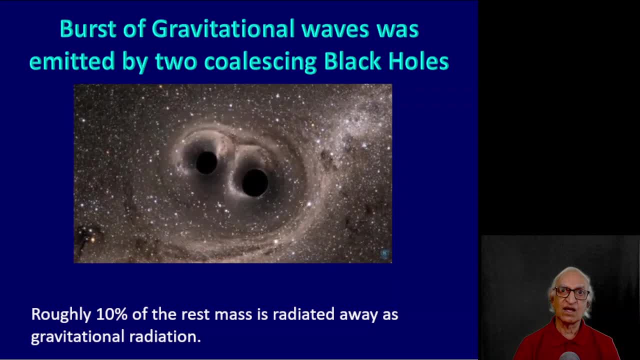 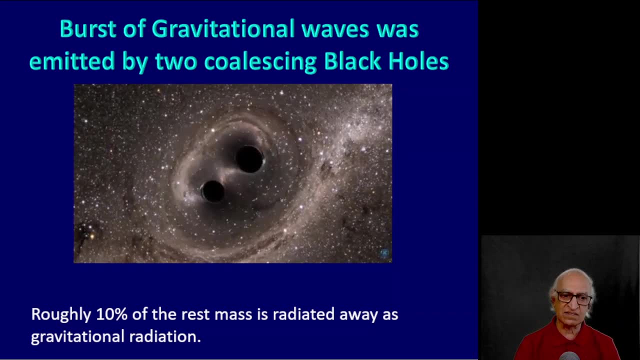 movement, a theokeness of gravitational shift, similar particles of incredible instant pulse, misschien C instruments of smoothizing theン- See Shakespeare fürs tiездes into a single black hole. In such a coalescence, roughly 10% of the 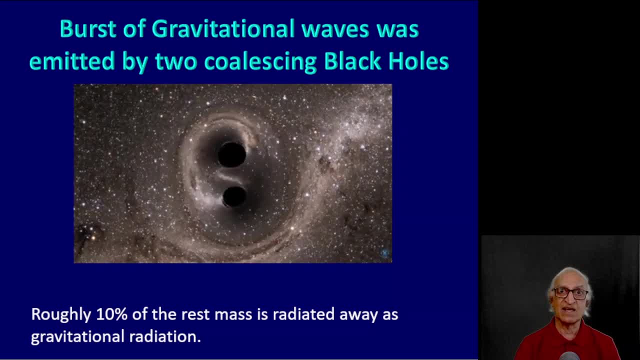 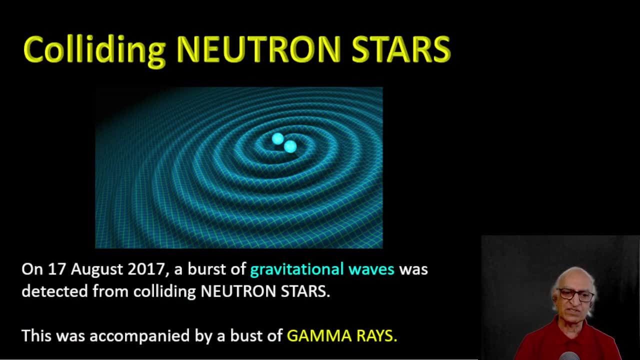 rest, mass energy of the black holes is radiated away as a burst of gravitational waves. Two years later, on 17th August 2017, a burst of gravitational waves was detected from colliding neutron stars. This particular burst of gravitational waves was also accompanied by a burst of gamma rays. What you see on the top. 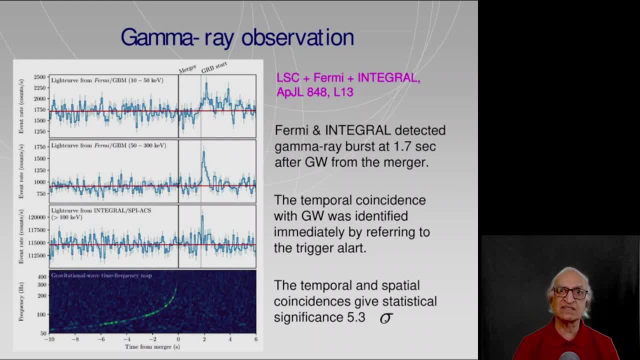 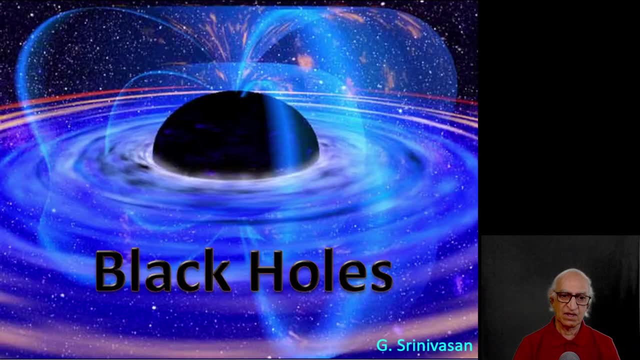 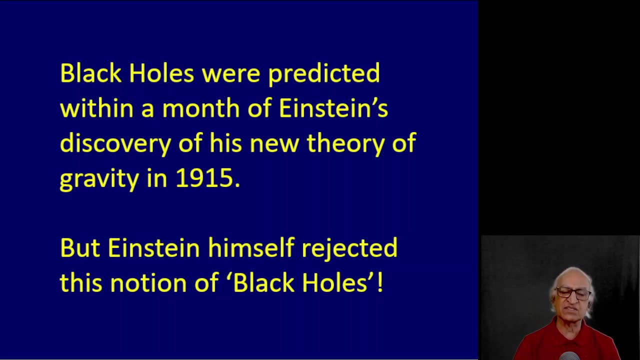 three panels is the gamma ray bursts at different energies. What you see in the bottom blue panel is the burst of gravitational waves, Black holes. Black holes are predicted within a month of Einstein's discovery of his new theory of gravity in November 1950.. 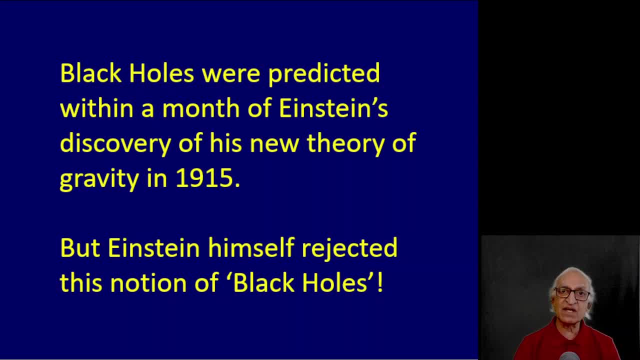 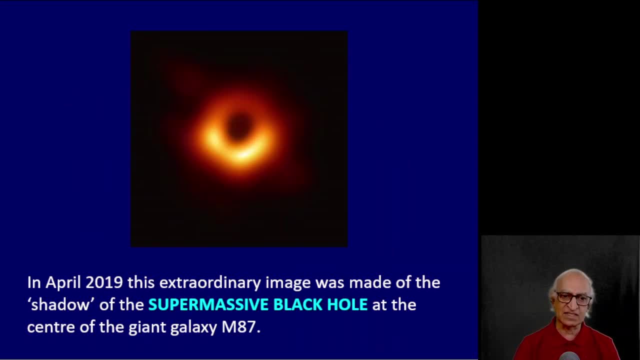 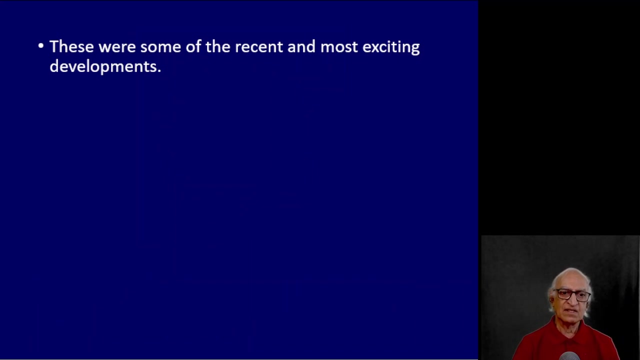 but Einstein himself rejected this notion of black holes. and yet, in April 2019, this extraordinary image was made of the shadow of a supermassive black hole at the center of a gigantic elliptical galaxy: M87. these were some of the recent and most spectacular developments in astronomy. 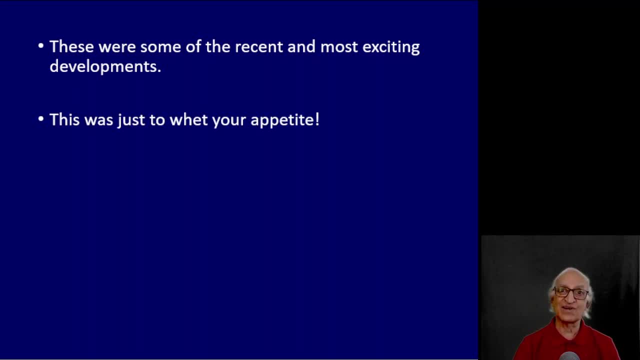 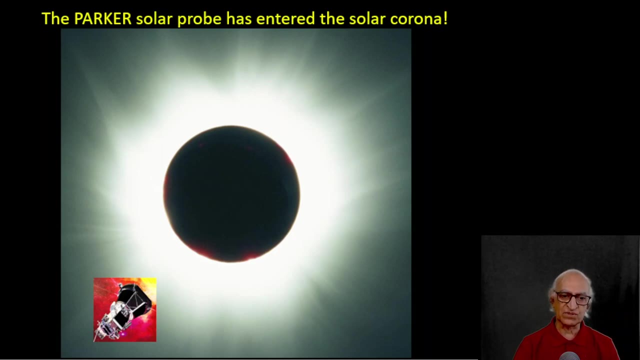 this was just to whet your appetite. you can look forward to sensational discoveries in the very near future. here is one. some years ago, NASA launched a satellite to probe the corona of the sun. it was named after the great astrophysicist Eugene Parker. 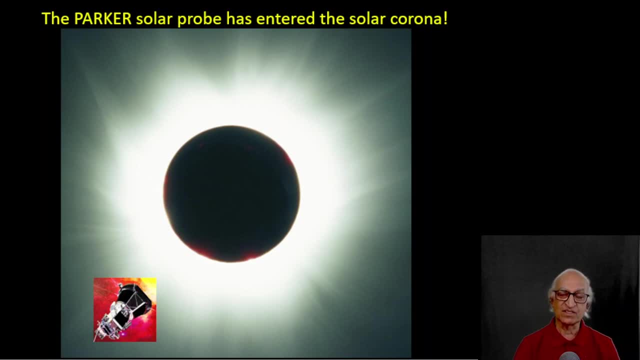 who passed away recently, a few days ago. The good news is that this satellite has now reached the Sun and it has entered the million-degree corona and has sent back valuable data successfully. It is expected that this satellite will orbit the Sun for the next four or five years. 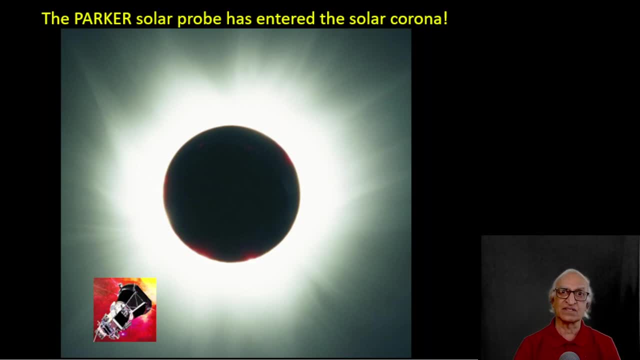 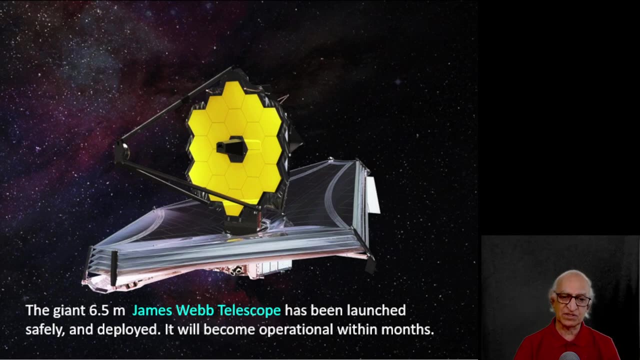 and we can hope to learn great many things about the secrets of the corona. The giant 6.5-meter James Webb Space Telescope has been launched, parked safely in its final parking place and has been deployed. Right now tests are going on of the alignment of the mirrors. 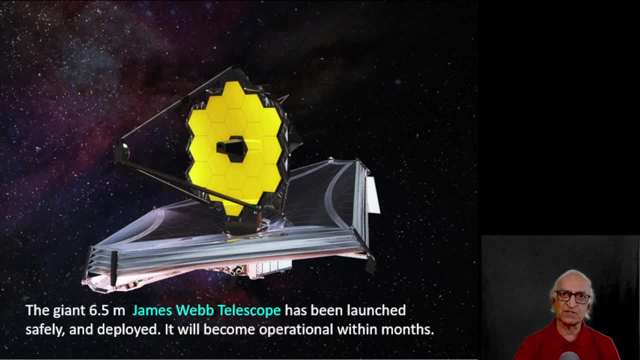 In the next couple of months it will take its first images. You all know the spectacular discoveries that the Hubble Space Telescope made. This is a far bigger and far superior telescope, and surely you can look forward to many spectacular and path-breaking discoveries. 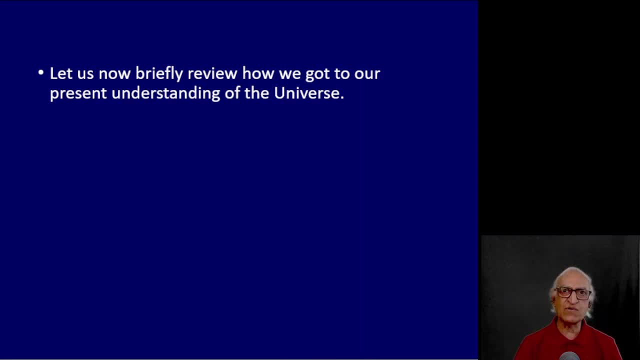 Let us now briefly review how we got to our present understanding of the universe. In this lecture, I shall not attempt to explain anything. This will be a fast-forward play of the revolution during the last 500 years. It is like visiting a fancy Michelin-starred restaurant and looking at the elaborate menu. 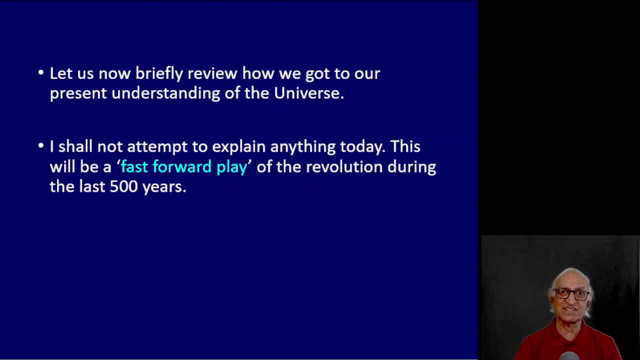 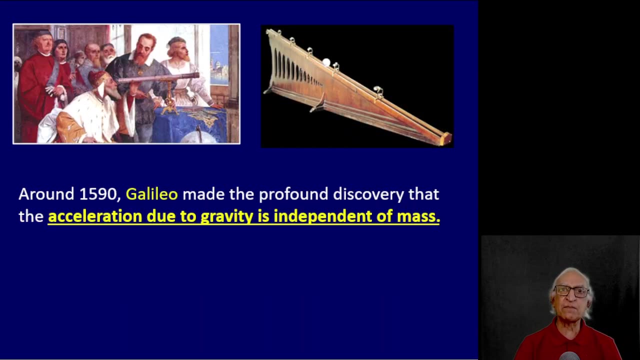 Today we will just look at the menu. We will revisit this restaurant and taste every dish on the menu. Similarly, in the lectures to follow, we shall systematically research every one of these momentous discoveries. We shall skip the great developments in antiquity. 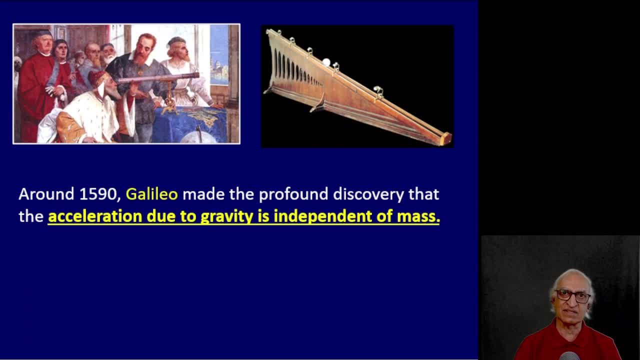 in Indian Vermilion неинг ceremony in India, ancient Greece, Mesopotamia and other countries and pick up the story around 1590, when Galileo did his famous experiments in the Leaning Tower of Pisa. In 1590, Galileo made one. 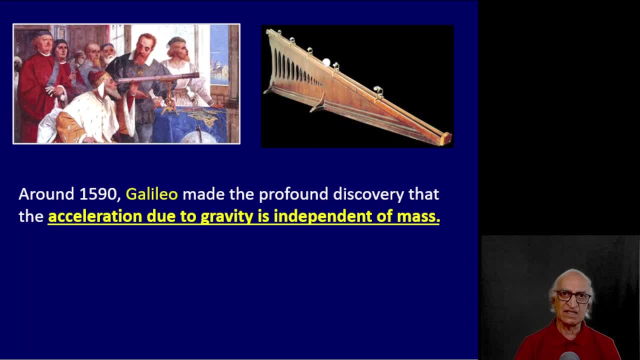 of the greatest discoveries in the history of physics. He demonstrated experimentally that the acceleration due to gravity is independent of the mass. Roughly 325 years later, Einstein advanced an explanation for this for the very first time. This explanation was at the base. 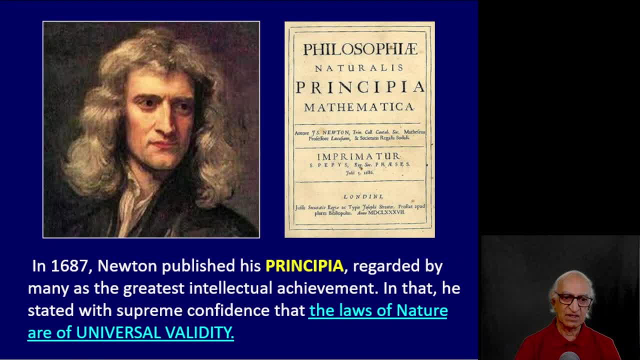 of his General Theory of Relativity. In 1687, Isaac Newton published his Principia, regarded by many as the greatest intellectual achievement. In that book he stated with supreme confidence that the laws of nature are of universal validity. What are the stars? 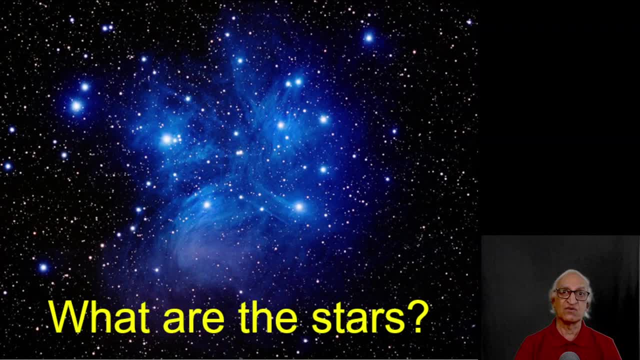 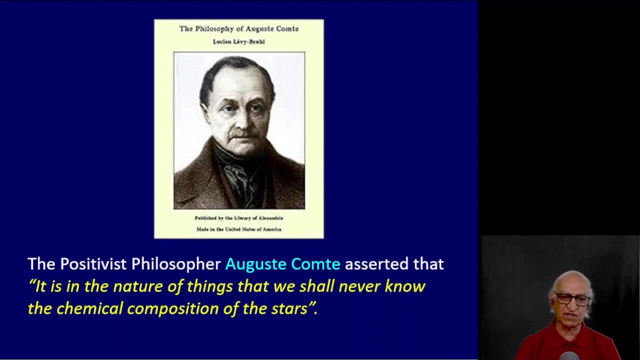 This question did not bother Galileo, Kepler or Newton, but this question was being asked in the 19th century. However, the positivist philosopher Auguste Comte, who was extremely influential in Western thinking, asserted that it is in the nature of things that we shall never know the chemical composition of the stars. 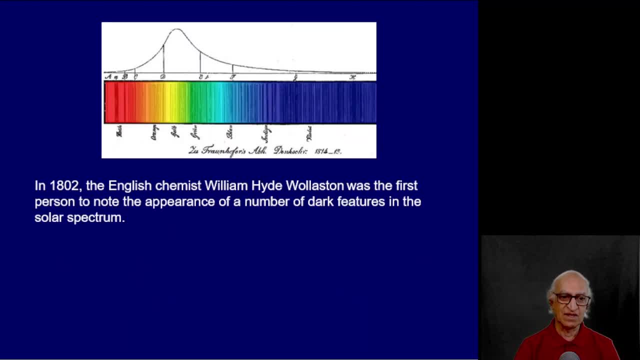 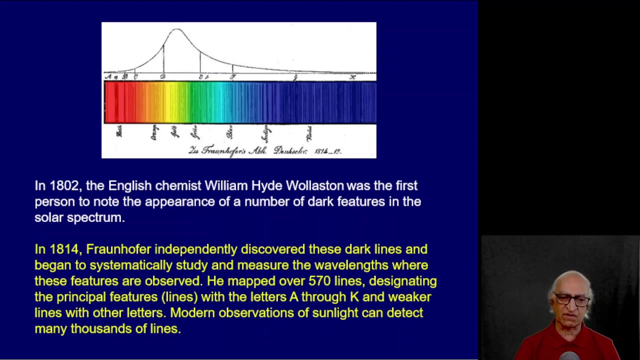 But soon it was proved wrong. In 1802 the English chemist William Wollaston discovered dark matter, Dark lines, in the spectrum of the sun. In 1814, young Fraunhofer in Germany independently discovered these dark lines and began to systematically study and measure the wavelengths where these 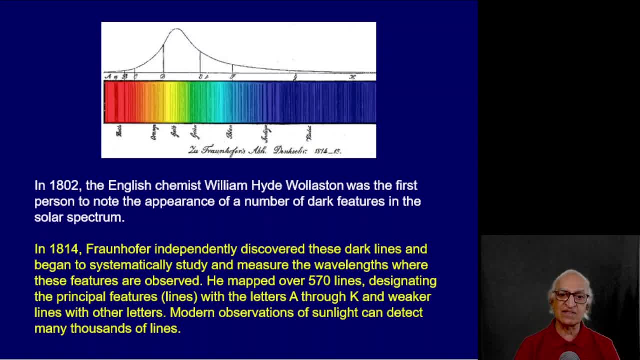 features are observed. He mapped over 570 dark lines, designated the principal features with the letters A through K and wicker them. he mapped over 570 dark lines, designated the principal features with the letters A through K and wicker them. 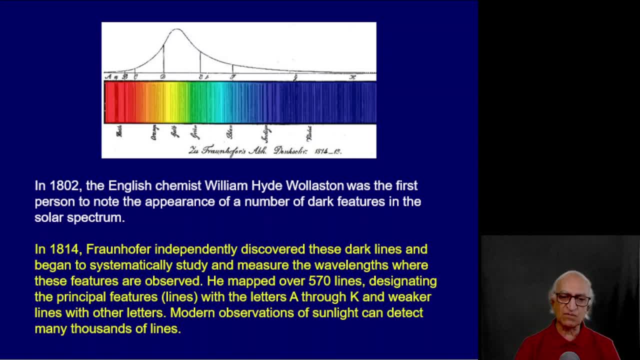 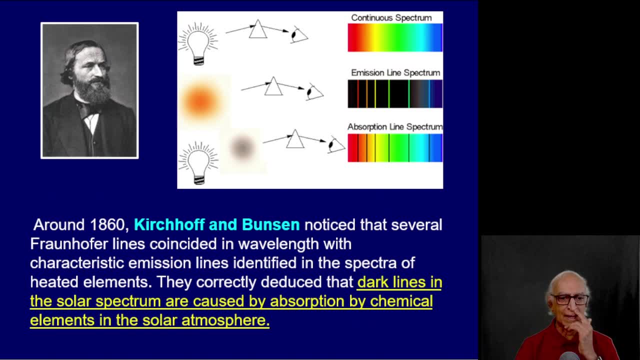 lines with many other letters. Modern observations of sunlight can detect many thousands of dark lines. Around 1860, the great German physicist Kirchhoff and Bunsen noticed that several Fraunhofer lines coincided in wavelength with the characteristic emission lines identified in the spectra. 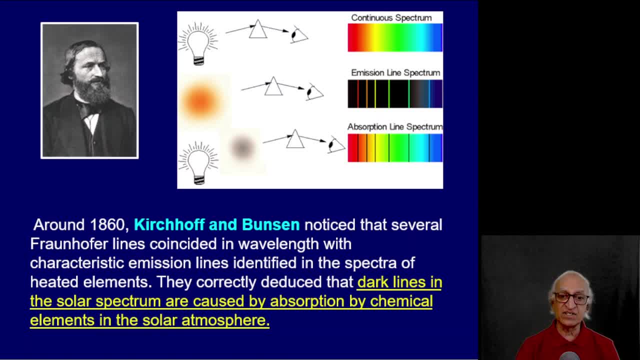 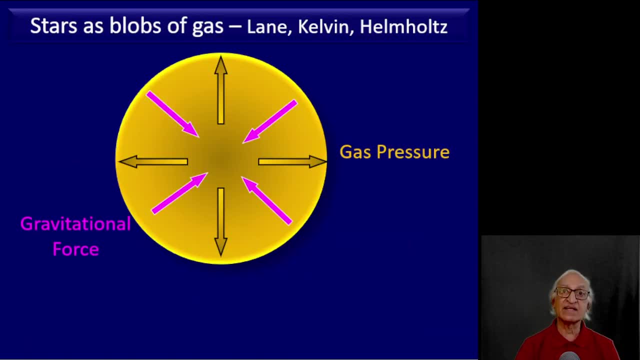 of heated elements. They correctly deduced that the dark lines in the solar spectrum are caused by absorption by chemical elements in the solar atmosphere, And a great revolution had begun. Lane, Kelvin, Helmholtz and others constructed a model of the stars as block globes of gas. 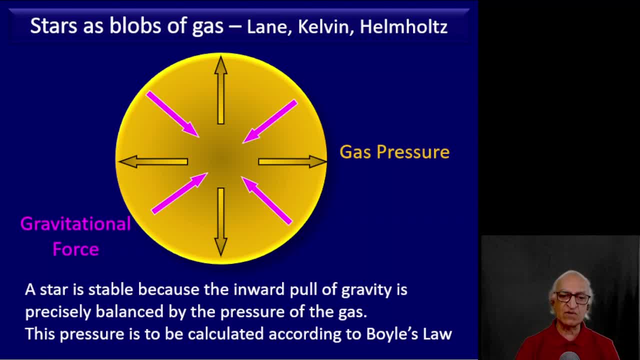 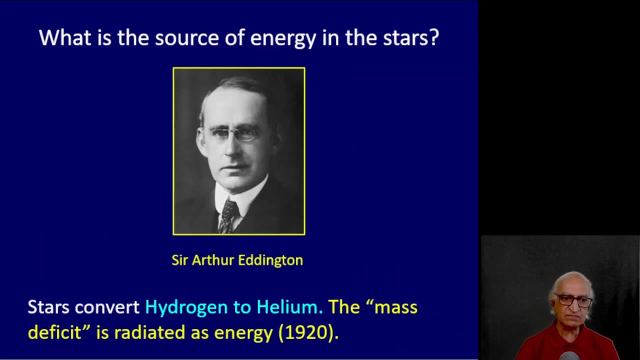 The said a star is stable because the inward pull of gravity is precisely balanced by the pressure of the gas. This pressure is to be calculated according to Boyle's law. This was their assertion. What is the source of the energy the stars radiate? 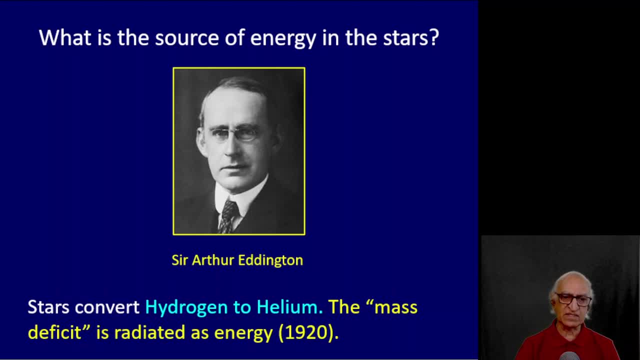 There are lots of theories at the time, but in 1920 Sir Arthur Eddington in Cambridge University made an extraordinary suggestion. He said that stars convert hydrogen to helium. He noticed that the mass of the helium nucleus was slightly smaller than the sum of the masses of four protons. 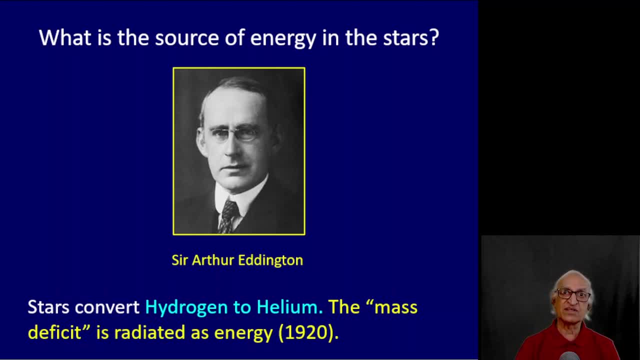 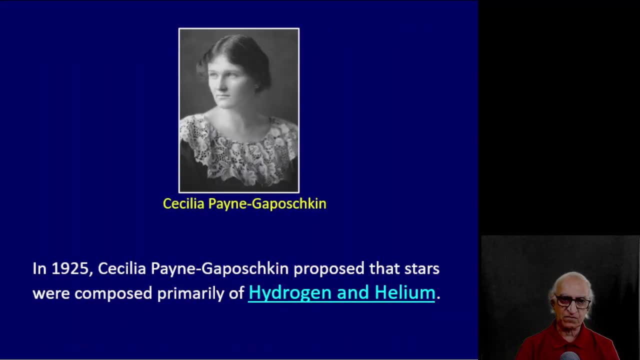 He said that this difference in mass is radiated away as energy, according to Einstein's EEE Equal to mc squared formula. What are the stars made of? Astronomers thought that at that time the stars are made up of heavy elements, like the earth is made up of heavy elements. A young student by name Cecilia Payne Kaposchkin. 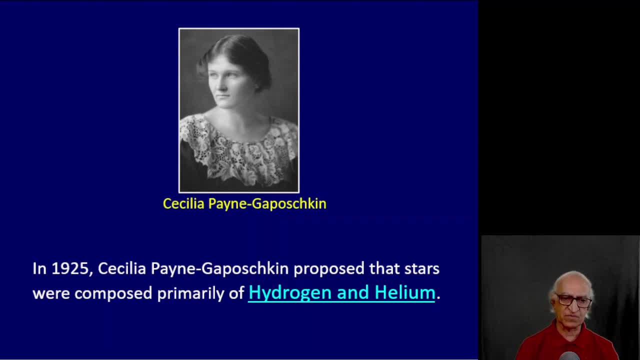 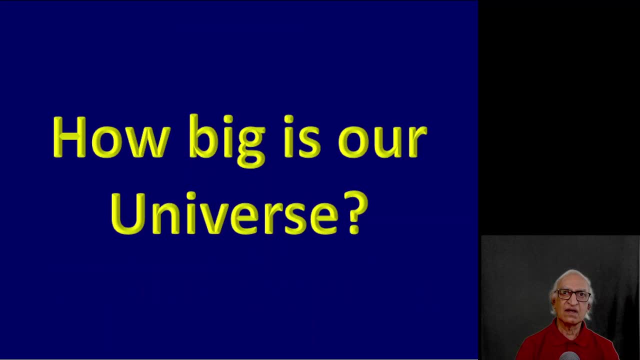 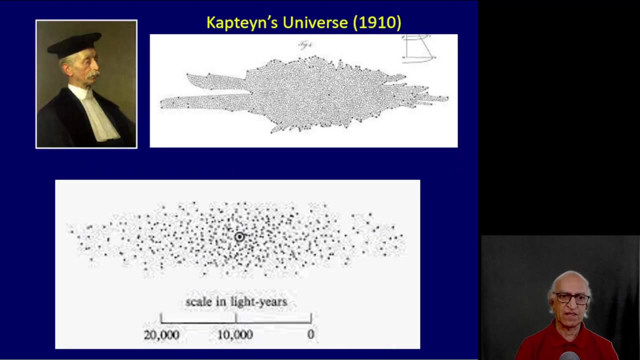 made an extraordinary suggestion in 1925 that the stars are made of heavy elements. The stars are made up of primarily hydrogen and helium. How big is our universe? This was another question at the dawn of the 20th century. The great Dutch astronomer Kapteijn decided to answer this question by measuring the position. 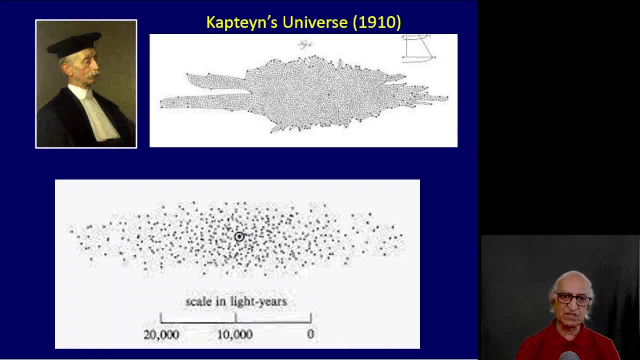 and distances to the stars in the sky, And the map that he made is shown in the upper panel. From this he constructed a model of the galaxy, which he said was the same as a model of the universe. The universe was rather small, just about a hundred thousand light years. 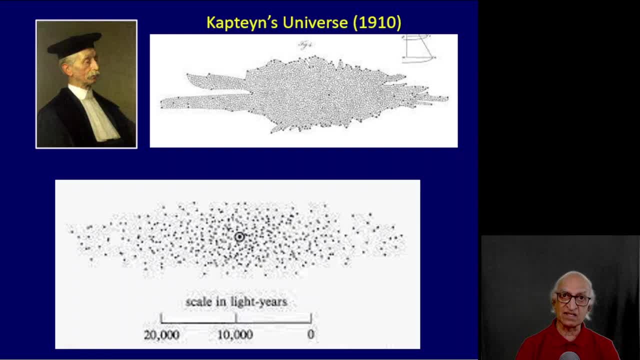 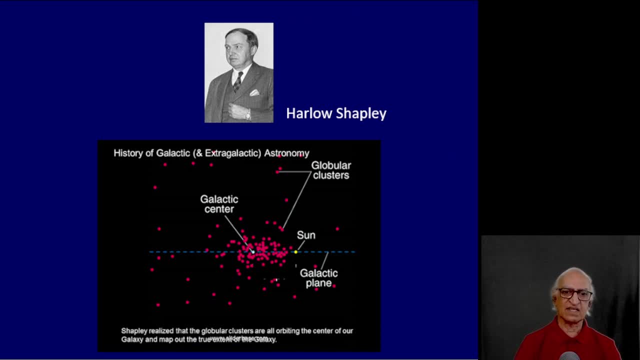 across. Most disturbingly, the sun was at the center of the universe. In the 1930s, the American astronomer Harlow Shapley in Harvard University measured the positions of globular clusters of stars And from that he deduced the dynamical center of our galaxy. 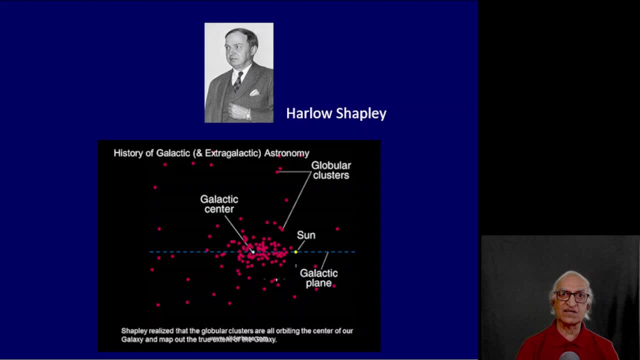 He discovered that this dynamical center of the galaxy, around which the globular clusters are going around in elliptical orbits, is not where the Sun is Indeed. the Sun was about 30,000 light years away from the center of our galaxy, And from this emerged the following picture of our galaxy. 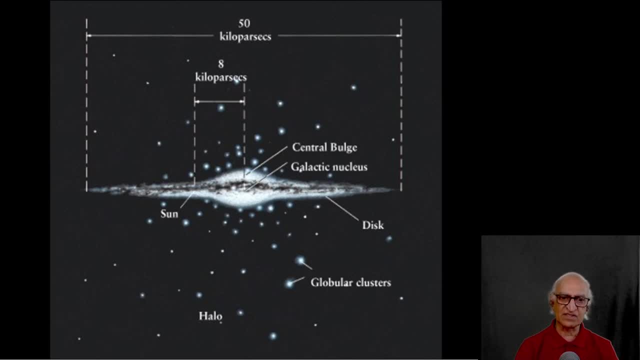 Our galaxy is a flattened disk with a central bulge. The globular clusters, the white dots that you see on the slides, are far away from the plane of the galaxy and they move around the center of the galaxy in elliptical orbits. 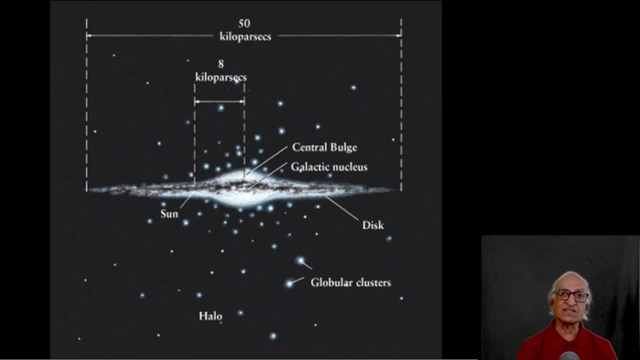 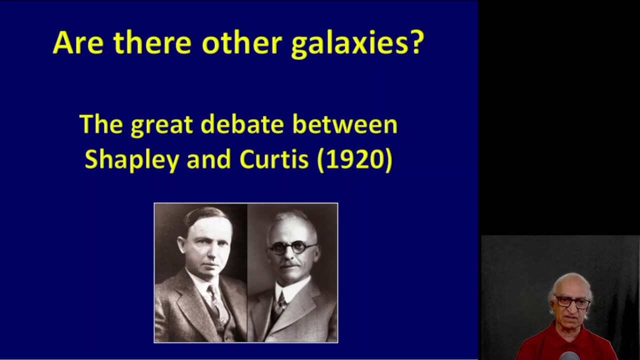 This model of our galaxy has survived the test of time. Another question at that time which was being hotly debated was: are there other galaxies? Is our galaxy the entire universe? In 1920, great public debate took place between Harlow Shapley and astronomer Curtis. 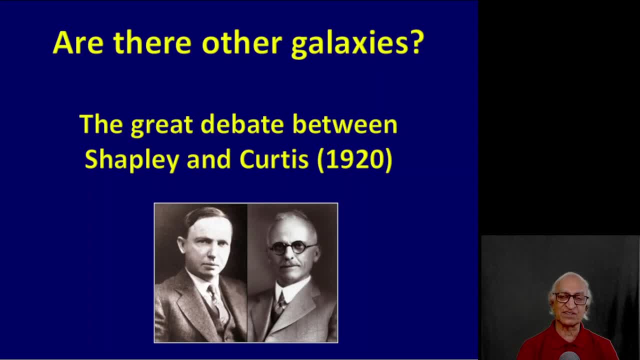 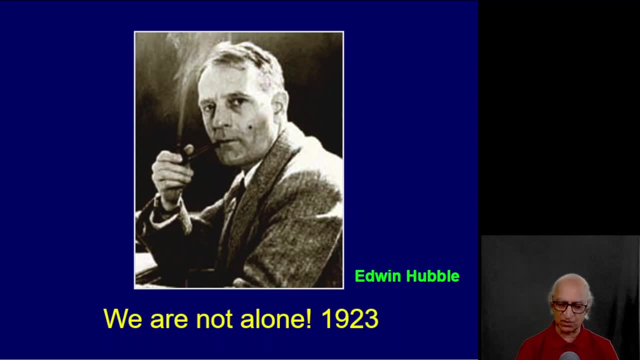 To settle this issue. the Hubble Space Telescope was a well-known astronomer and the Hubble Space Telescope was a well-known astronomer, But they couldn't settle this issue. But the issue was settled soon after that, in 1923, by the great American astronomer Edwin Hubble. 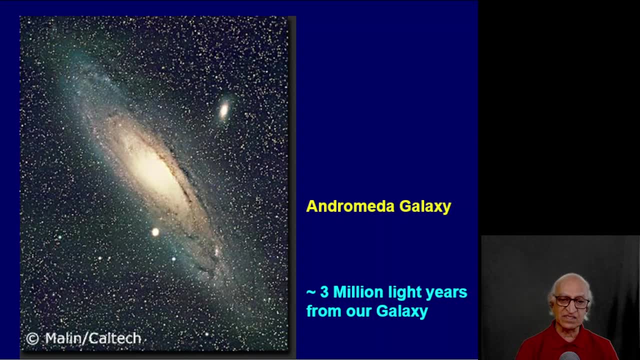 Hubble demonstrated that we are not alone. He did this by measuring the distance to the Andromeda Galaxy. Contrary to what was thought before, the Andromeda Nebula was not inside our galaxy, but away from our galaxy at a distance of about 3 million light-years. 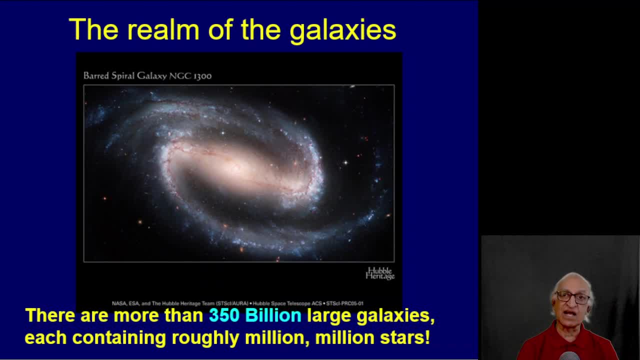 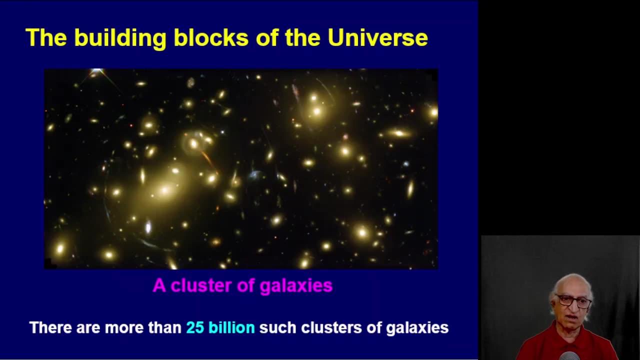 And soon it became clear that it was a realm of galaxies. Today we know that there are more than 350 billion large galaxies, each containing a million million stars, And, as I said before, they're building blocks of our universe, or clusters of galaxies. 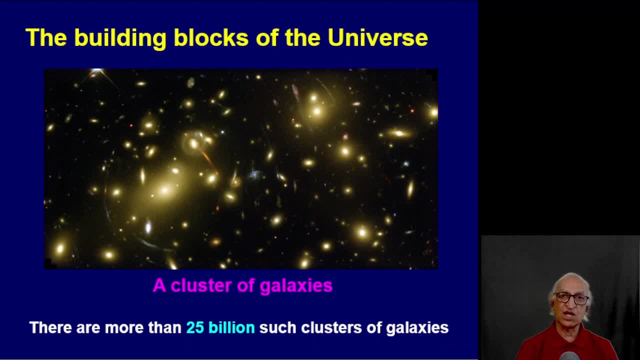 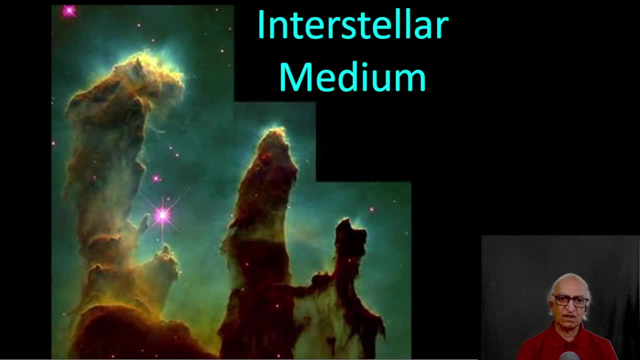 such as the one that is shown in this slide, such as the one that is shown in this slide, such as the one that is shown in this slide, and there are more than 25 billion such clusters of galaxies. What is there between the stars? 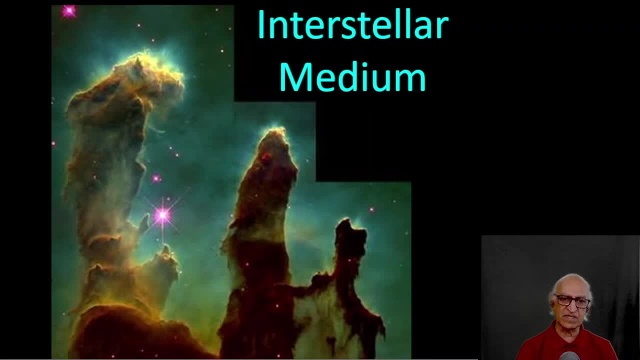 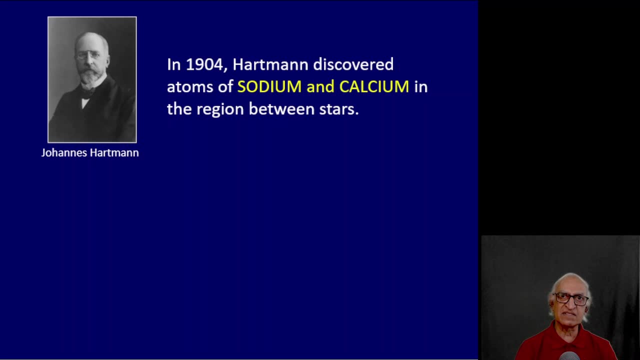 It was demonstrated that there is an interstellar medium. This came about in the following way: In 1904, the Argentinian astronomer Hartmann discovered atoms of sodium and calcium. discovered atoms of sodium and calcium in the space between the stars. 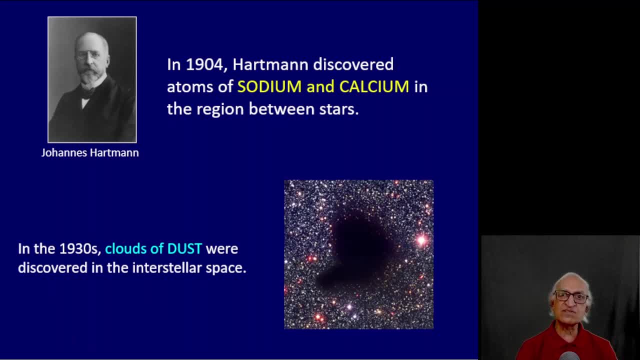 In the 1930s, clouds of dust were discovered in interstellar space. In the 1930s, clouds of dust were discovered in interstellar space. Where there is dust, there must be gas, And thus emerged the interstellar medium. 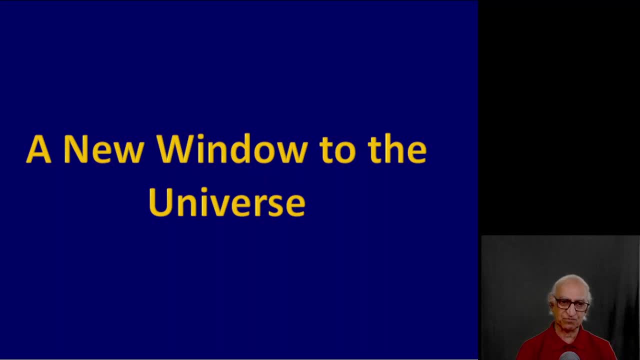 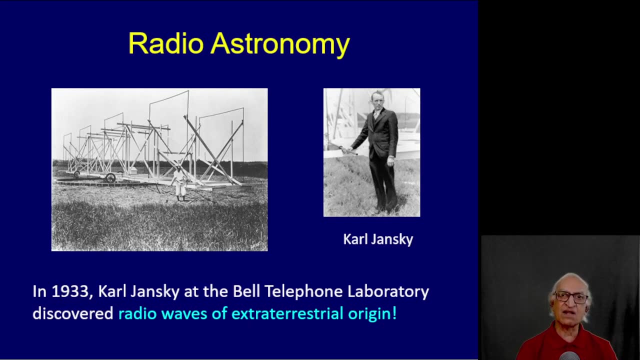 We shall speak about that at length during these lectures. We shall speak about that at length during these lectures. A new window to the universe. A new window to the universe In 1933, Carl Jansky working at the British University. 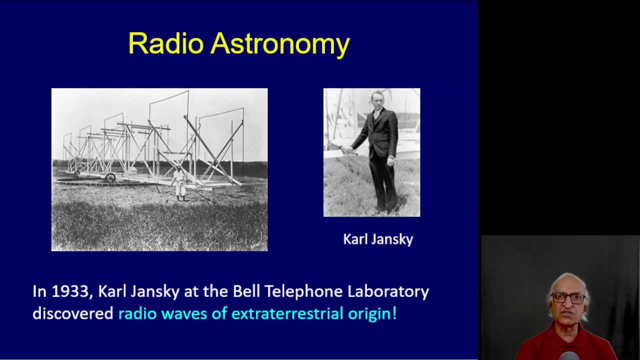 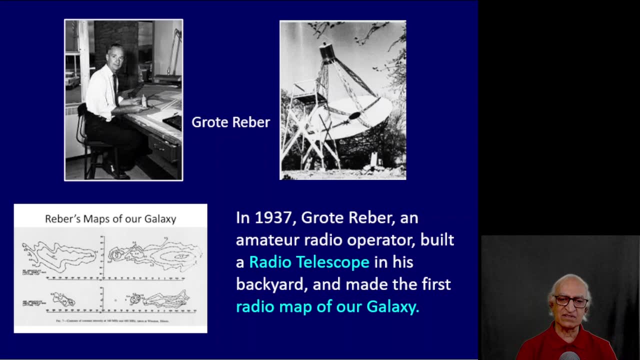 in the Bell Telephone Laboratory discovered radio waves of extrasolar origin. discovered radio waves of extrasolar origin In 1937, Grote Reber, an amateur radio operator- an amateur radio operator, a hand- built a radio telescope in his own backyard. 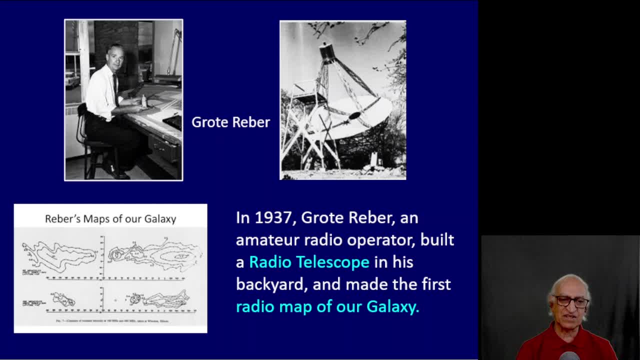 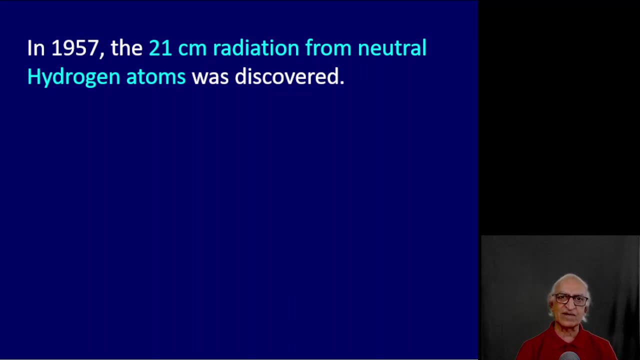 with his own money and made the first radio map of our galaxy. and made the first radio map of our galaxy, which you see on the left hand side panel, which you see on the left hand side panel. In 1936,, In 1957, one of the greatest discoveries was made in astronomy: the discovery of the 21-centimeter radiation from neutral hydrogen atoms. 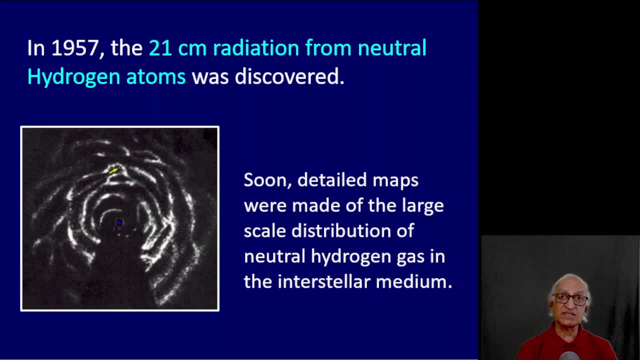 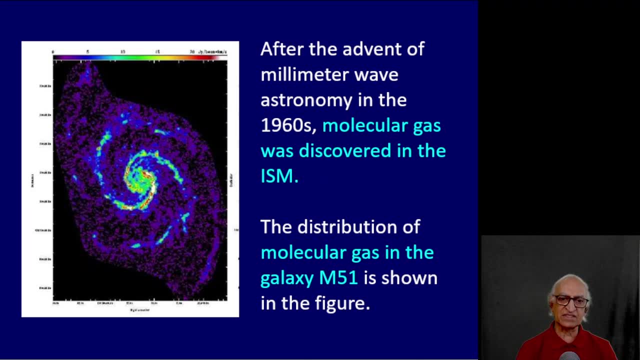 Soon, detailed maps were made of the large-scale distribution of neutral hydrogen gas in the interstellar medium. In the 1960s, with the advent of millimeter-wave astronomy, molecular gas was discovered in the interstellar medium. In this picture you see the distribution of carbon monoxide gas in the galaxy M51.. 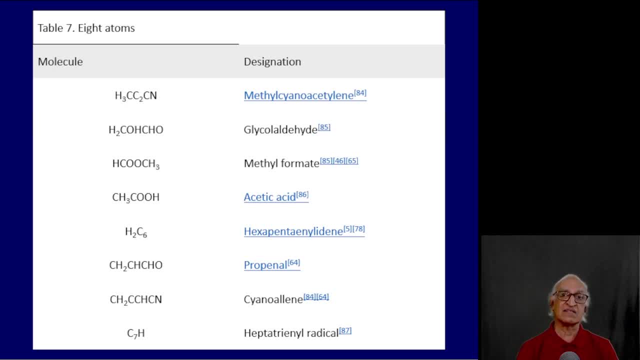 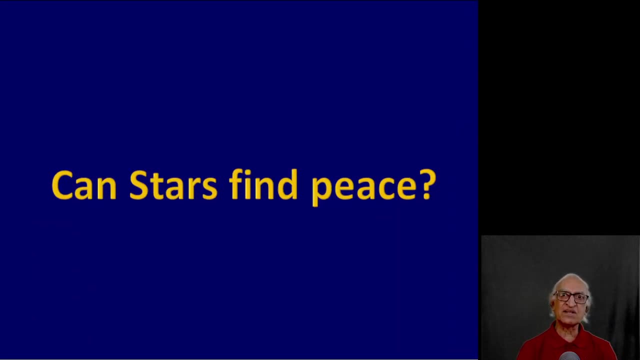 Today, astronomers have discovered hundreds and hundreds of molecules in the interstellar region. Some of them are in the interstellar medium. Some of them are extremely complicated molecules. Here is a sample of a few of the complicated molecules. Can stars find peace? 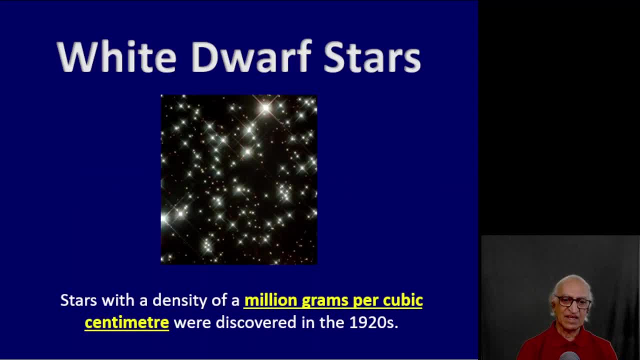 What does it mean with that question? In the 1920s, stars with a density of a million grams per cubic centimeter were discovered. For your reference, the average density of the sun is just a little over the density of water. It is 1.4 grams per cubic centimeter. 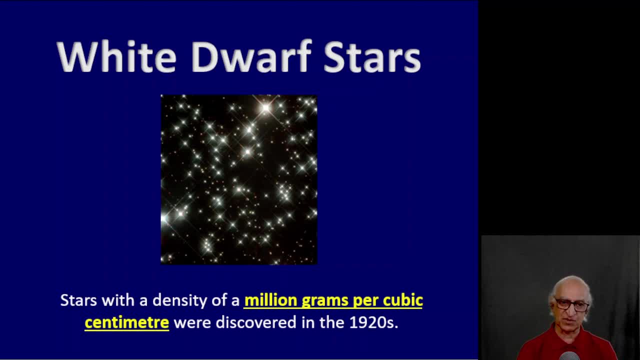 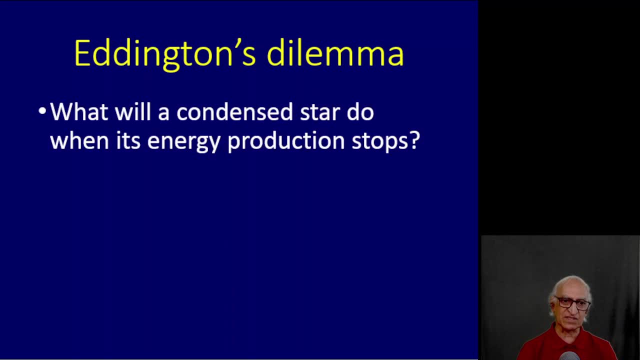 But the density of these stars was a million grams per cubic centimeter. This made Eddington extremely alarmed. He asked the question: what will a condensed star do when its energy production stops, when its nuclear reactor at the center fails? Will it collapse to a point due to gravity? 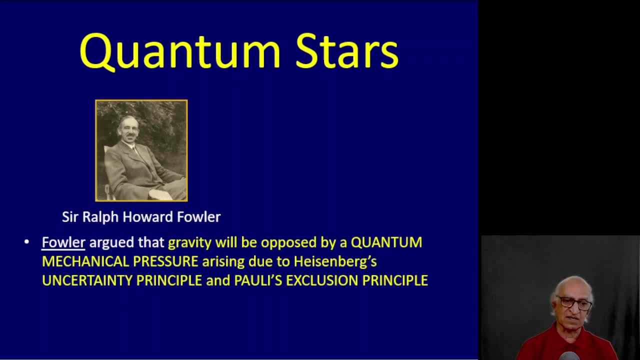 Well, this question was. This question was answered in an ingenious manner by Sir Ralph Fowler, a colleague of Eddington at Cambridge University. Fowler argued that gravity will be opposed in these stars by a quantum mechanical pressure, a pressure that arises due to the combined effect of Heisenberg's uncertainty principle and Pauli's exclusion principle. 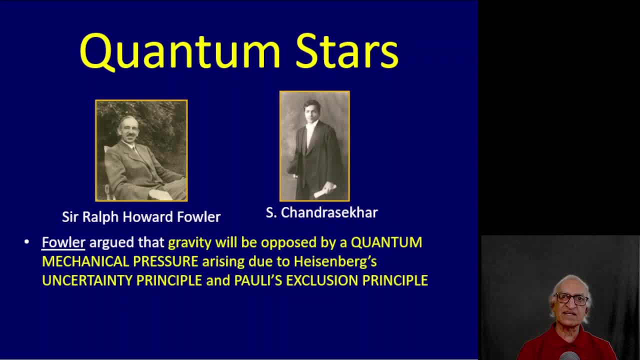 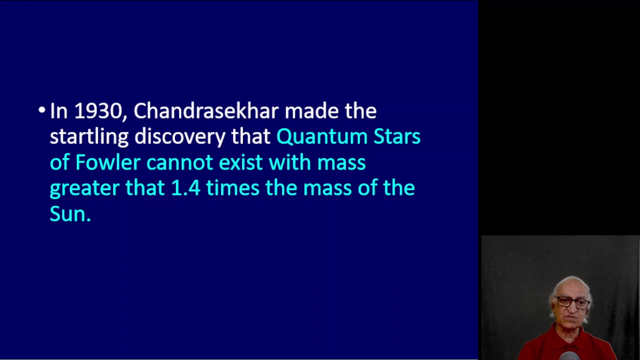 Young said. Subramanian Chandrasekhar, a second year Bsc student at Presidency College in Madras, went on to construct a detailed theory of such quantum stars based on Ralph Fowler's suggestion. In 1930, Chandrasekhar made the startling discovery that quantum stars of Fowler cannot exist with masses greater than 1.4 tons. 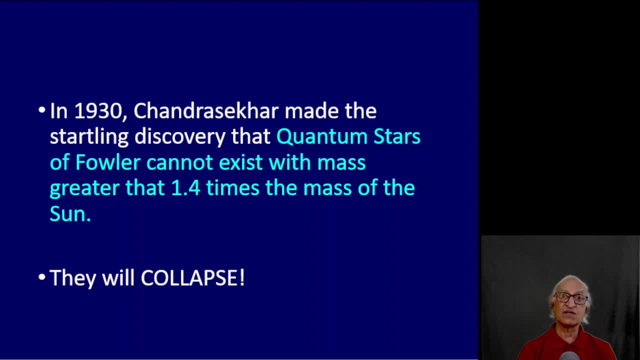 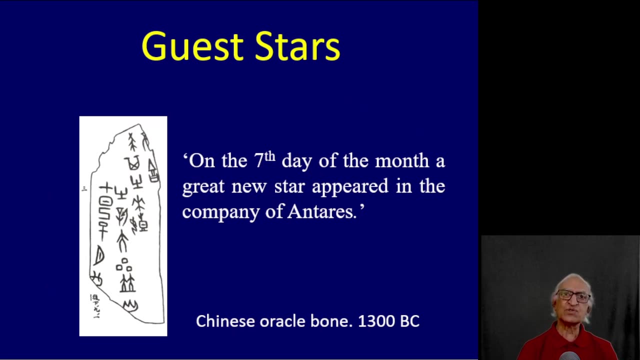 the mass of the Sun, They will collapse. This represented nothing less than the overthrow of the Aristotelian principle of the cosmos. Every now and then, a new star appears in the sky. The Chinese called them guest stars. They shone for a 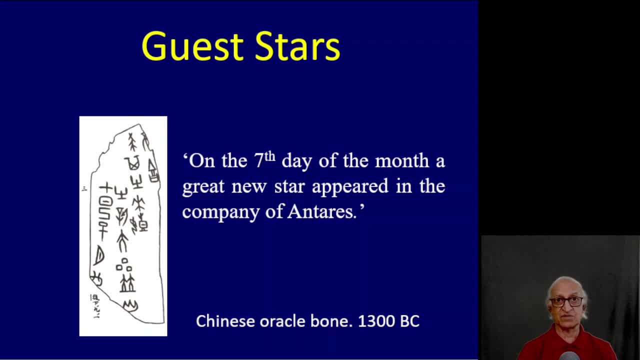 few days, sometimes a few months, sometimes even a year. Then they faded away. For example, in 1300 BC, the Chinese astronomers have written: on the seventh day of the month a great new star appeared in the company of Antares. 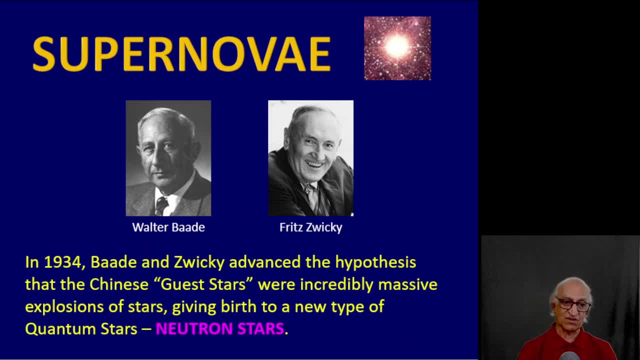 What are these guest stars? Well, no one knew. In 1934, two astronomers of the California Institute of Technology, Walter Bardet and Fritz Zwicky, advanced the extraordinary hypothesis that the Chinese guest stars were incredibly massive explosions of stars giving birth to a new type of quantum stars- neutron stars. In 1938 and 39, Robert Oppenheimer and his students at Berkeley University, University of California at Berkeley, were able to discover a new type of quantum star. They showed that there is a limiting mass to neutron stars also, just as there is a 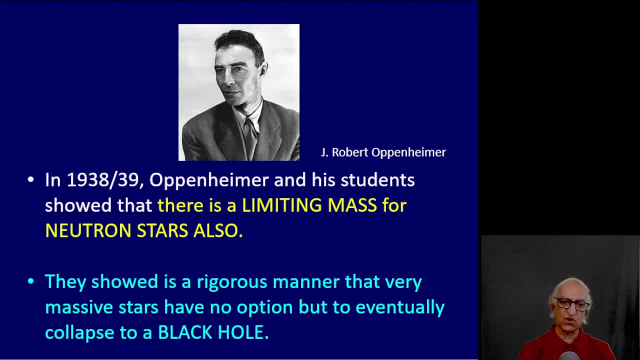 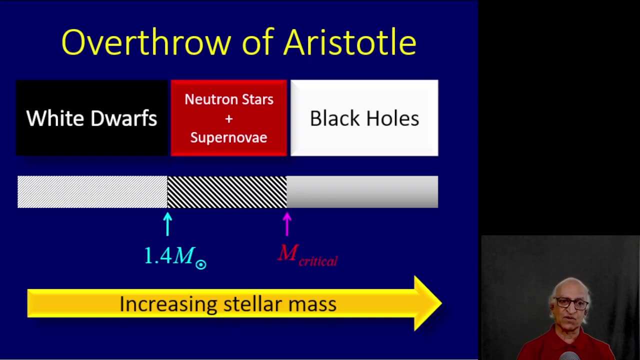 limiting mass to white dwarf stars. They showed in a rigorous manner that very massive stars have no option but to eventually collapse to black holes. So the overthrow of Aristotle Aristotelian philosophy was complete. The final nail in Aristotle's sword was the one that was cut off from the star. 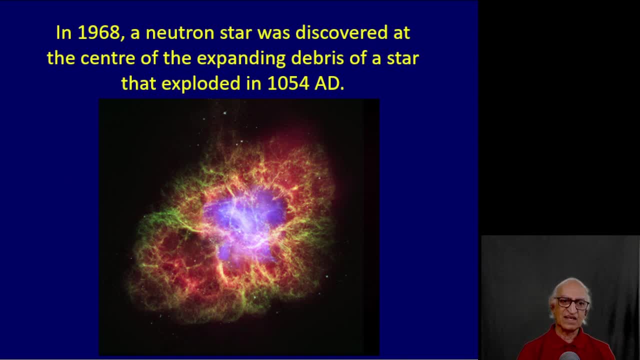 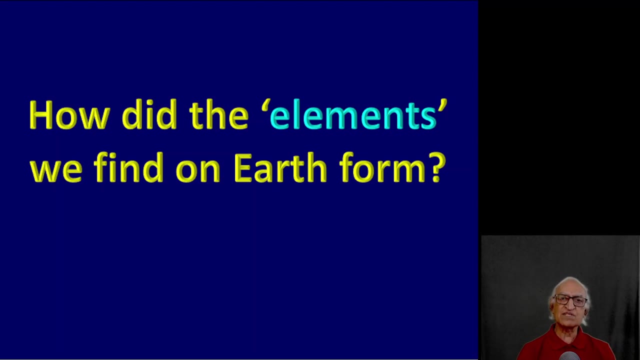 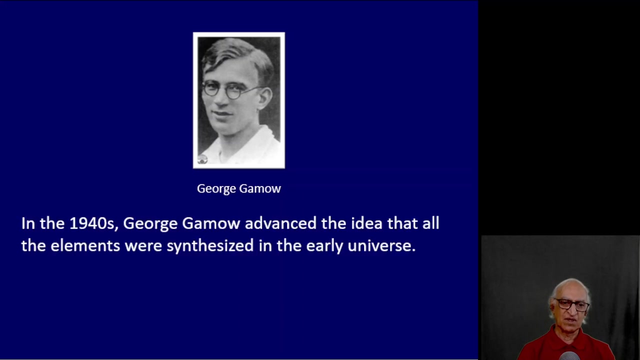 Aristotle's coffin came in 1968.. A neutron star was discovered at the center of the expanding debris of a star that exploded in 1054 AD. How did the elements we find on the earth form? A brilliant young theoretical physicist by name George Gamow advanced the idea in the 1940s that all the elements were. 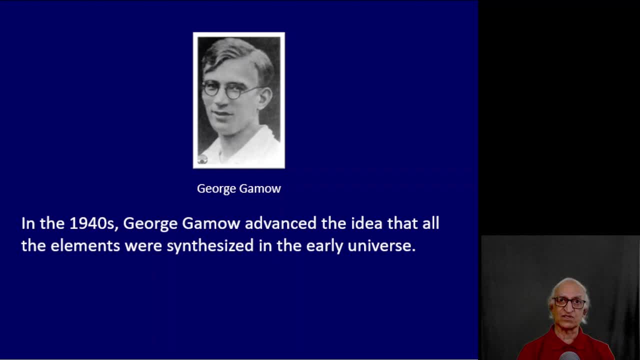 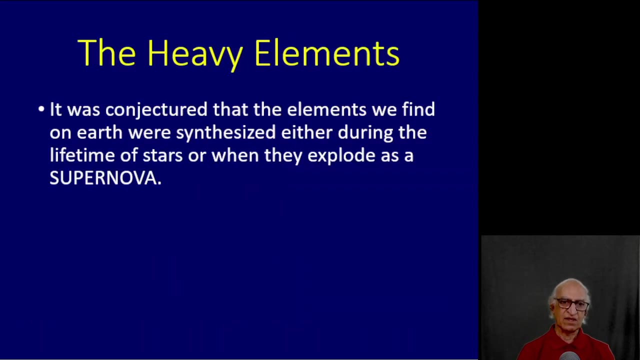 synthesized in the very early universe, when the universe was extremely hot and extremely dense. Detailed calculations showed that deuterium, helium and some lithium were in fact synthesized in the early universe. It was conjectured that the elements we find on earth were synthesized not in the early universe but in stars either, during the lifetime of the stars. 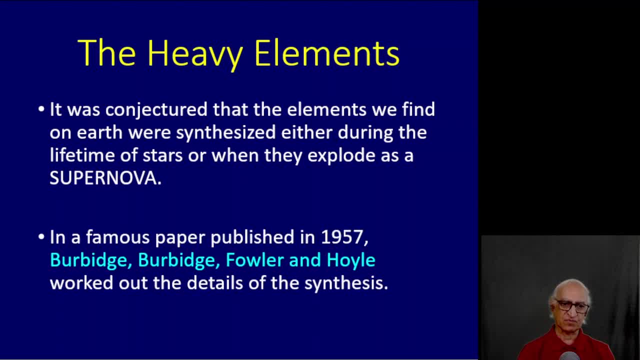 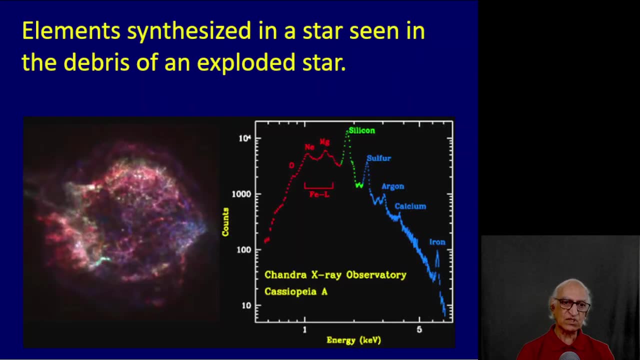 or when they explode as a supernova explosion. In a famous paper published in 1957, Berg, Land, Bergwitz, downer and Hoyle worked out the detailed theory of nucleosynthesis in stars, What you see in the picture on the left. 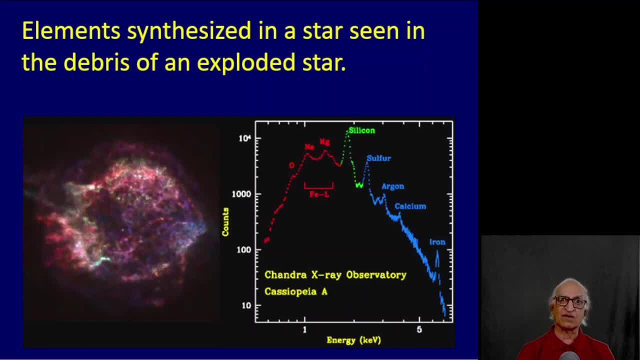 is the debris- expanding debris- of the star that exploded about 300 years ago. this is an X-ray image, a image taken by BJZ Project in 1931- and the expand debris in around the world. This is a X-ray image. an image taken by BJZ Project in 1931 and the expand debris in around the world. an image taken by BJZ Project in 1931 and the expand debris in around the world. This is an X-ray image, an image taken by BJZ Project in around the world. 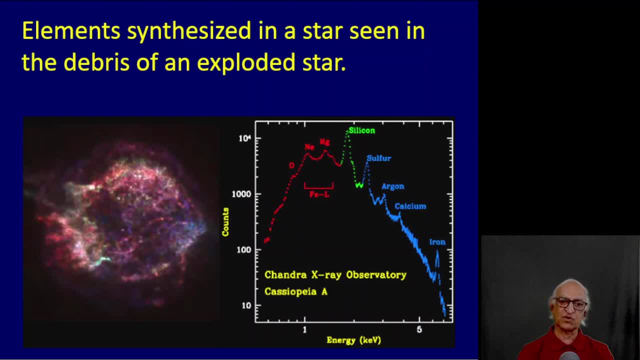 with an X-ray telescope, and the X-ray telescope is the great Chandra X-ray Observatory. What you see on the panel on the right is the spectrum of X-rays from this expanding debris, And there you see elements synthesized in the stars and during the explosion. 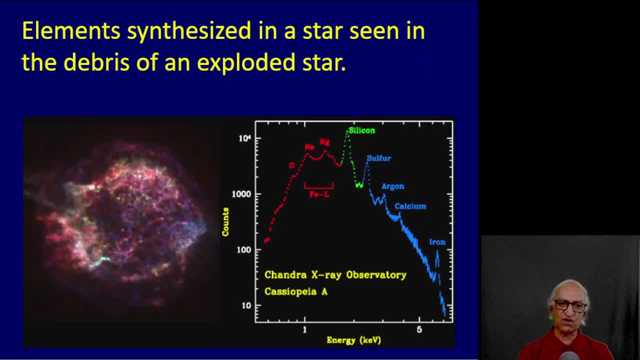 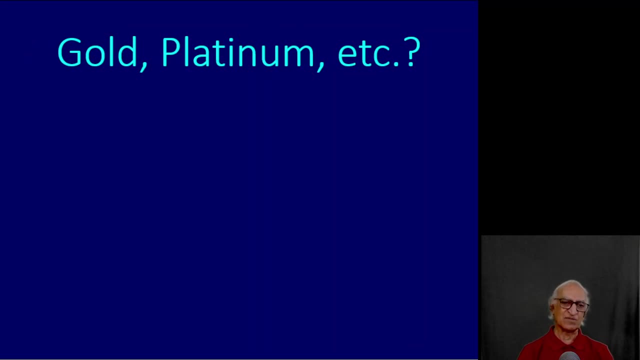 You see very clear signature of oxygen: neon, magnesium, silicon, sulfur, argon, calcium, iron and so on. What about gold, platinum and other exotic elements? There were difficulties in synthesizing these elements, either during the lifetime of the 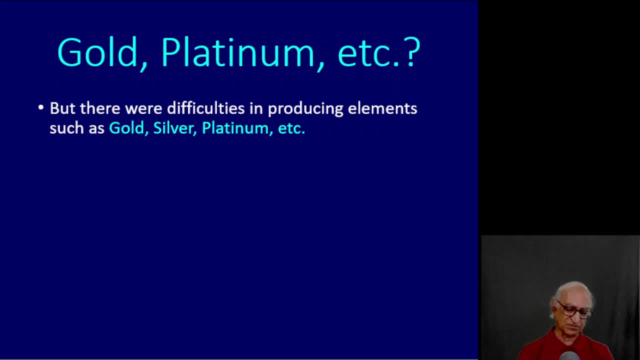 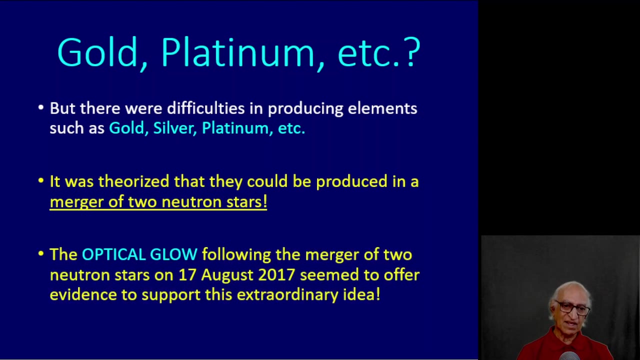 stars or even during stellar explosion. An extraordinary suggestion was made many years ago that these elements- gold, platinum, et cetera- could be synthesized in two neutrons. The first is that the stars and the neutron stars merge, The optical globe which followed the gravitational wave burst and the gamma ray burst on 17 August. 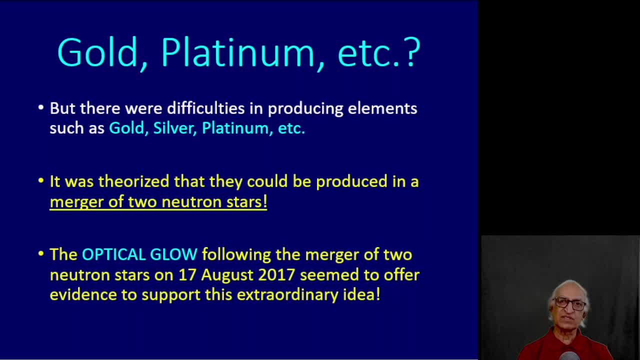 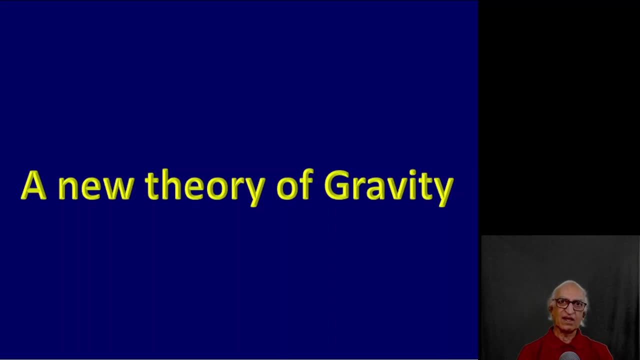 2017, seemed to offer evidence to support this extraordinary idea. The dust hasn't settled down on this. The jury is still out on the exciting possibilities: A new theory of gravity? Soon after Einstein's special theory of relativity in 1905, it became clear that Newton's theory 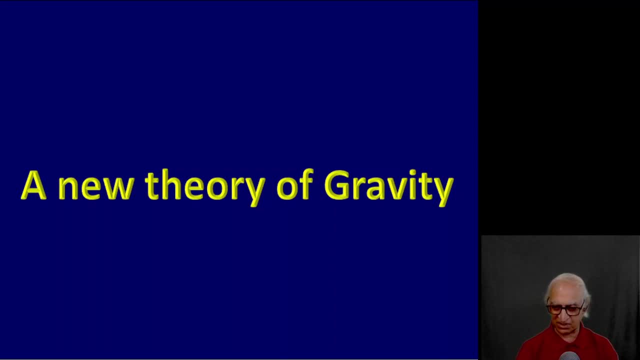 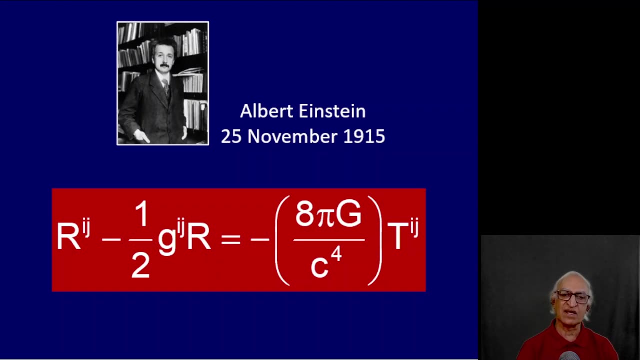 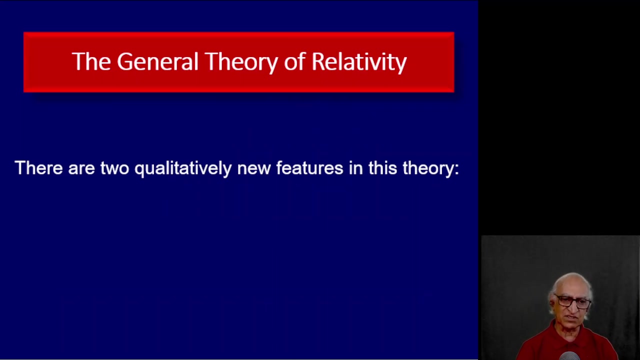 of gravity was not consistent with the special theory of relativity. On the 25th of November 1915, Einstein published his new and revolutionary theory of gravity, The general theory of relativity as it is called. It had two new qualitative features which weren't there in Newtonian gravitational theory. 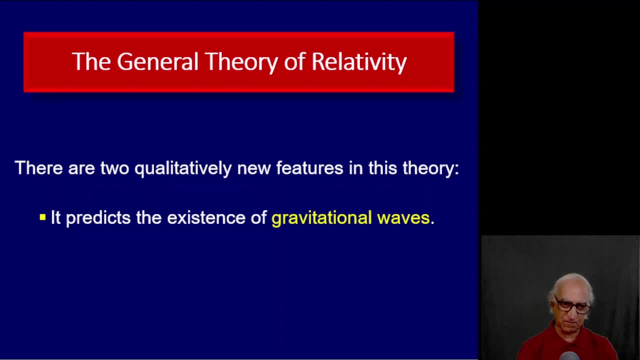 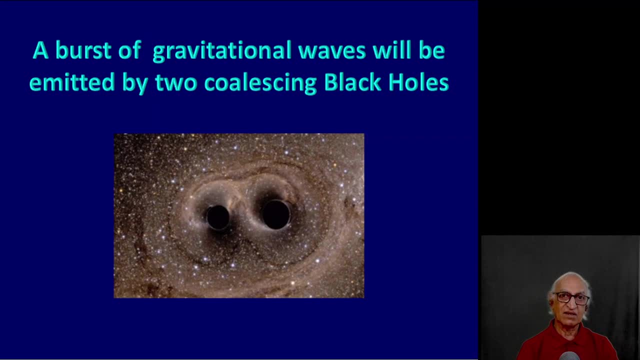 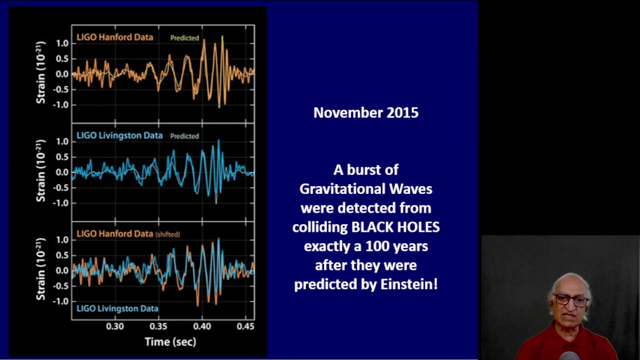 First, it predicted the existence of gravitational waves. Second, it predicted the occurrence of black holes. For example, if two black holes spiraled in and eventually coil us, the theory predicts that there will be a burst of gravitational waves. As I said before, in November 2015, a burst of gravitational waves was detected and the 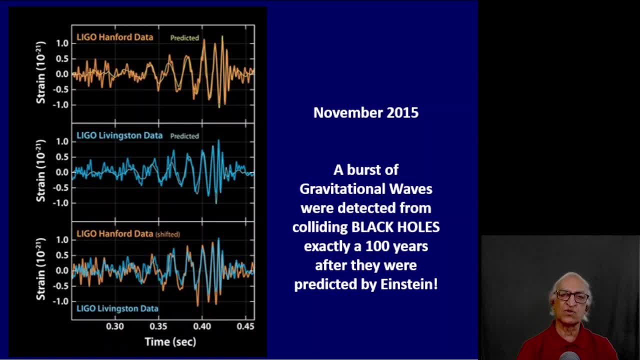 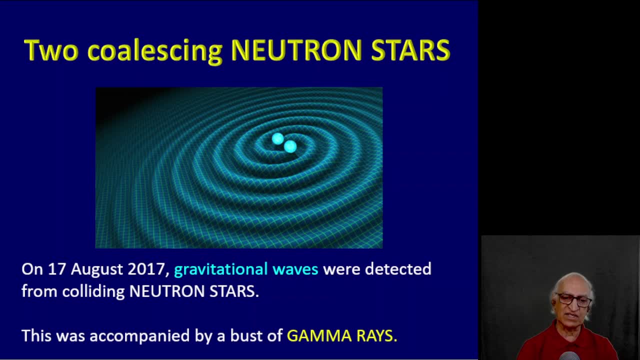 signature of this burst clearly pointed to two black holes coalescing. On 17 August 2017, gravitational waves were detected from colliding neutron stars. Again, as I said in the beginning, this was accompanied by a burst of gamma rays. 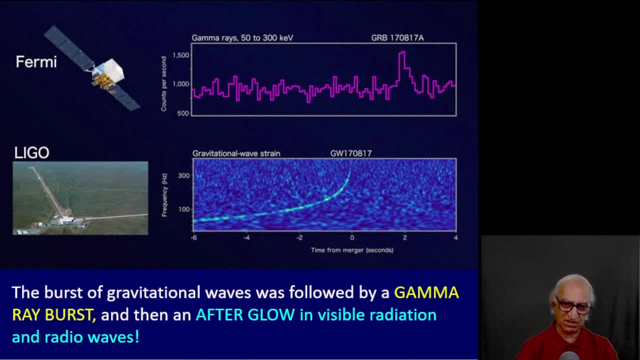 This was the first time that gravitational waves were detected from colliding neutron stars. This was the first time that gravitational waves were detected from colliding neutron stars. What you see on the right-hand side of the top panel is the burst of gamma rays and 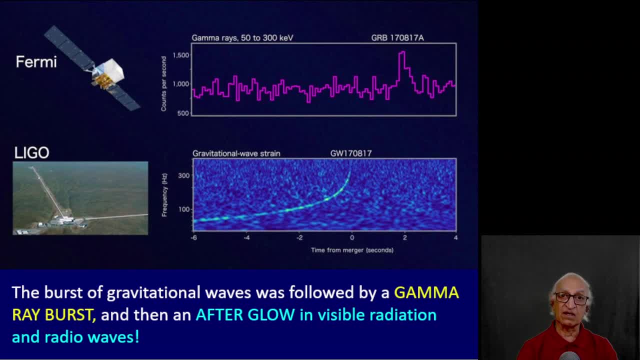 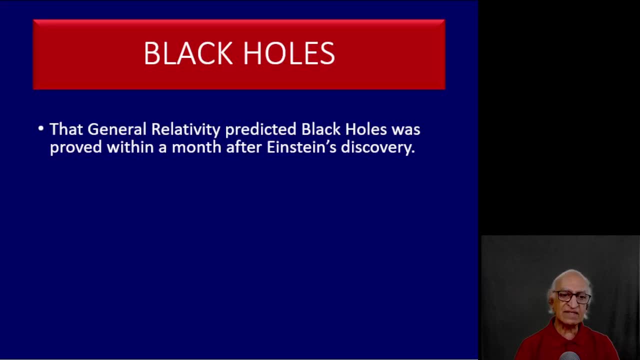 what you see below in the blue panel is the burst of gravitational waves. That general theory of relativity predicted black holes was proved by the great German physicist Karl Schwarzschild within a month after Einstein's discovery of the theory of gravitational gravity. The remarkable discoveries by Chandrasekhar in 1932 and by Oppenheimer and his student. 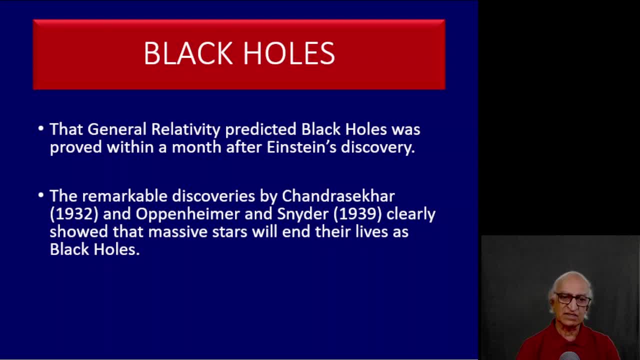 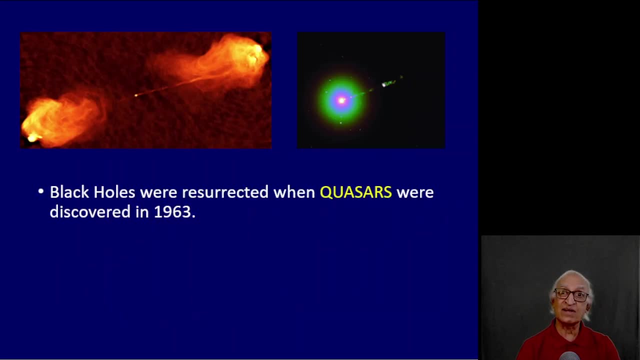 Schneider in 1939 clearly showed that massive stars will end their lives as black holes, But this notion was summarily rejected by physicists, most notably by Einstein himself. Black holes were resurrected when quasars were discovered. They used to be called black holes. 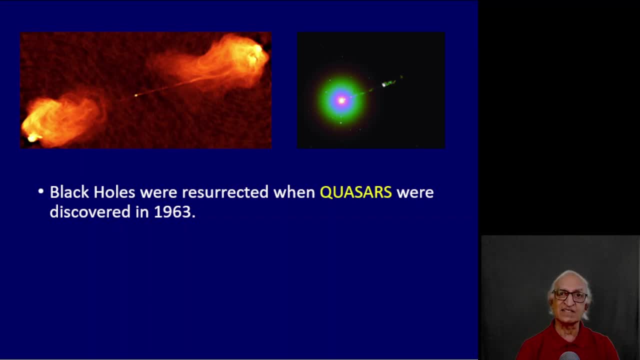 Black holes were used to create black holes. Black holes were used to create black holes. Black holes were used to create black holes. Black holes were pulled from these black holes. Black holes were pulled from these black holes. Black holes were pulled from these black holes. 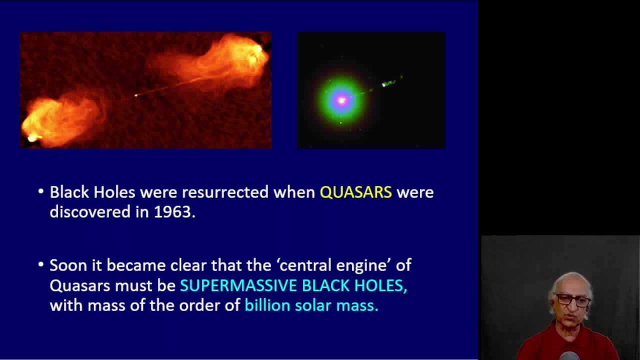 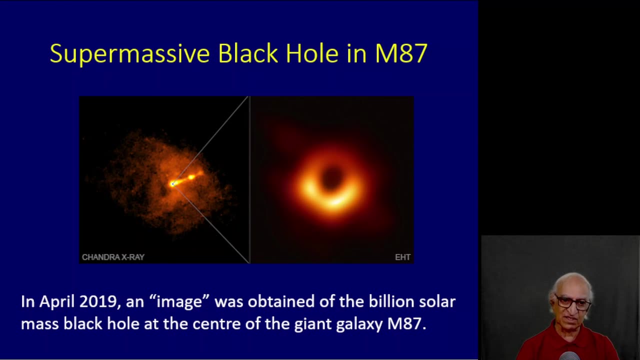 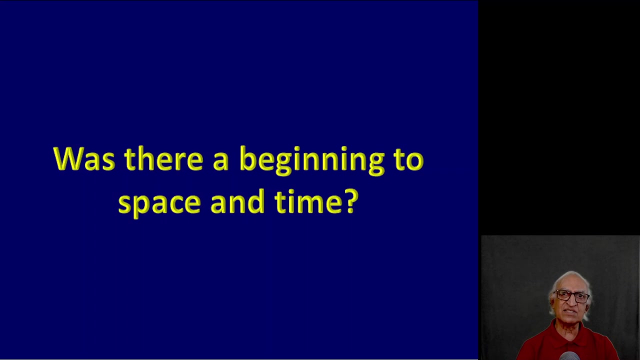 They vibrated at anaran as been whether the one that the컨 was on the left. It was the punchle, the conscious brain. But no one, even inpatients, invented these things of the elliptical galaxy in 87.. One of the grandest questions of all time is: was there? 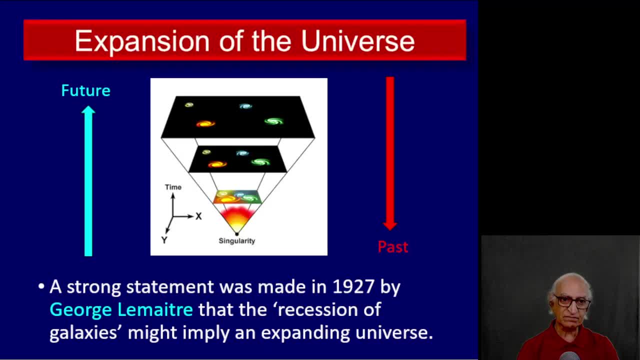 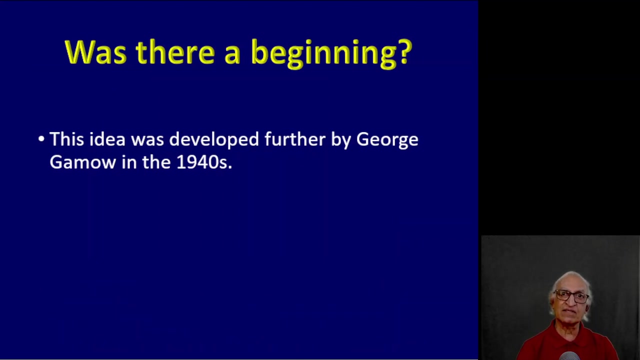 a beginning to space and time itself. A strong statement was made in 1927 by George Lemaître, a Catholic priest in Belgium. He conjectured that the recently discovered recession of galaxies might imply an expanding universe. This idea was developed further by 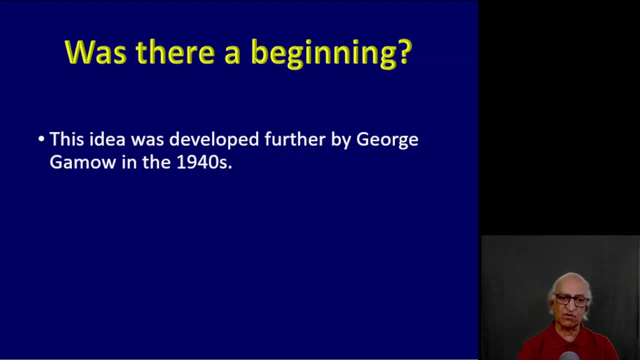 the Russian physicist George Gamow in the 1940s. But the question- was there a beginning? remained meaningless till the 1960s. It remained meaningless because the question could not be posed in a rigorous manner within the premise of science. 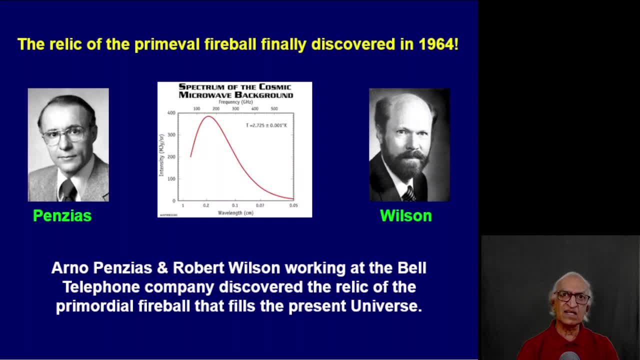 George Gamow had conjectured that the early universe must have been very dense and very hot and that the relic of this primeval fireball must still be there in the universe. This relic of the primeval fireball was discovered in 1964 by Penzias and Wilson working at the 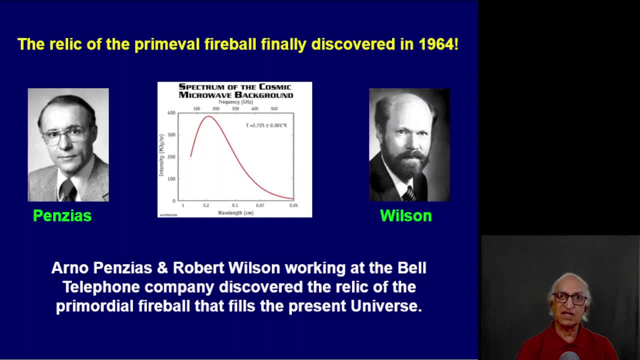 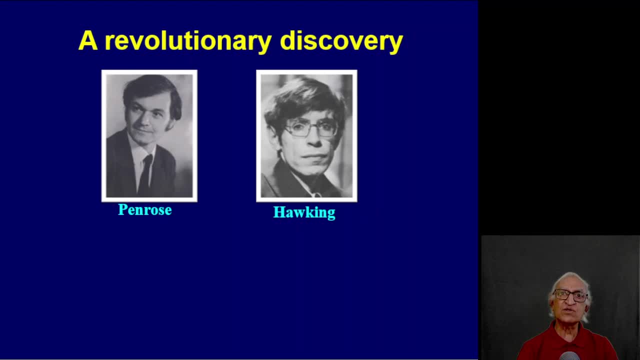 Bell Telephone Laboratory. This is the Cosmic Microwave Background Radiation. Soon after that, a truly revolutionary discovery was made by Roger Penrose and Stephen Hawking. In a series of singularity theorem, they obtained a revolutionary result Stated in simple terms. according to them, the universe could have begun from. 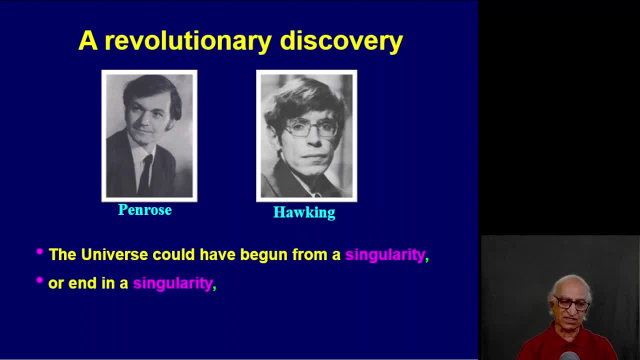 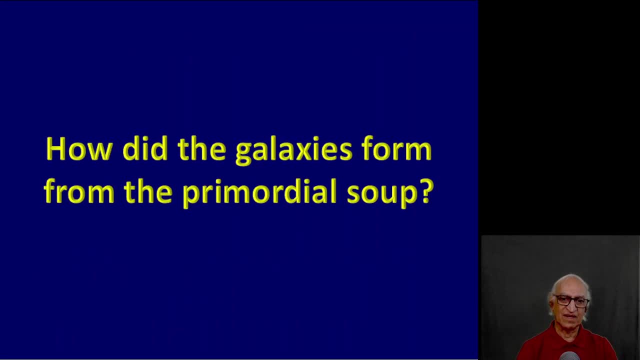 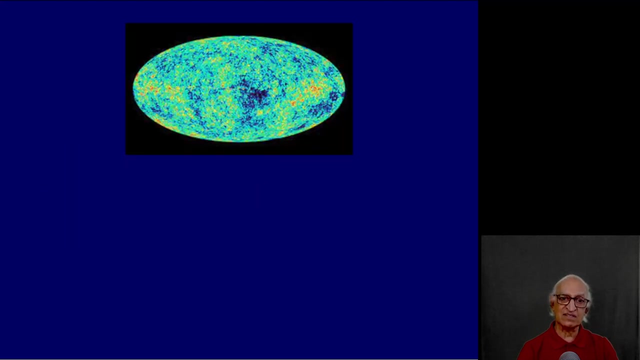 a singularity or end in a singularity, or both began and will end in a singularity. If the early universe was highly dense, hot and a homogeneous primordial soup, how did the galaxies form? It was discovered in the 1980s that the Cosmic Microwave Background Radiation was 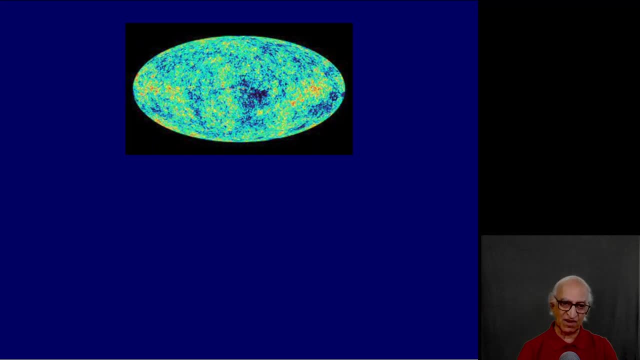 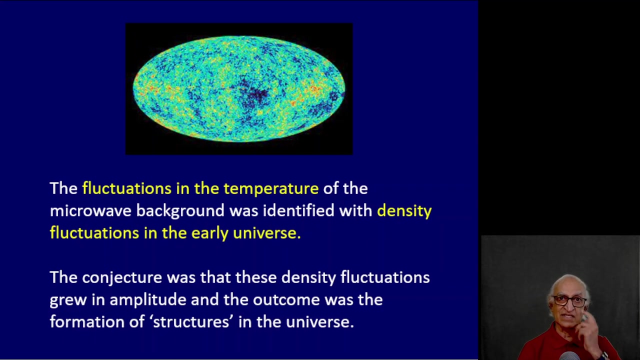 not uniform in temperature. everywhere There were fluctuations in the temperature. These fluctuations were identified with fluctuations in the density of matter in the early universe. So the conjecture was that these density fluctuations grew over a period of time, and that is how structures appeared in the universe such as we see now. 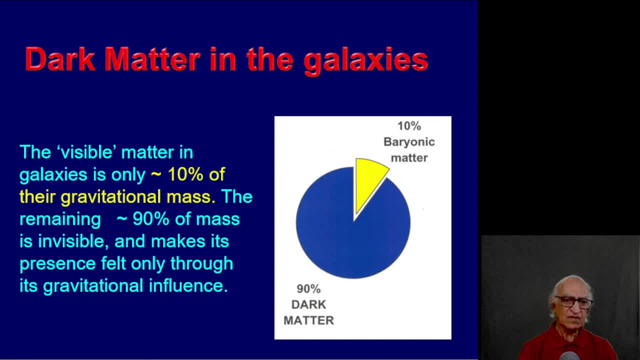 In the 1980s and 1990s it emerged from detailed astronomical observations that visible matter, matter of the kind that we are made of, constitutes only 10% of the gravitational mass of galaxies. It was demonstrated experimentally extremely convincingly that 90% of the mass of galaxies 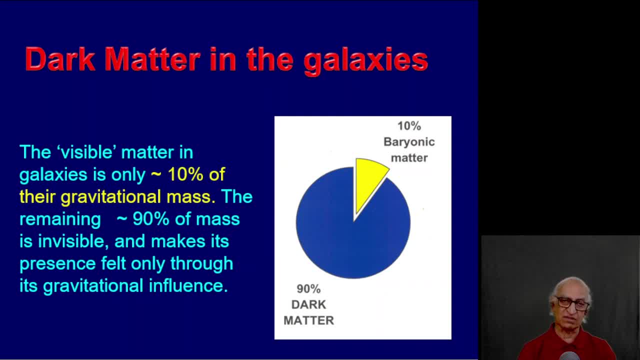 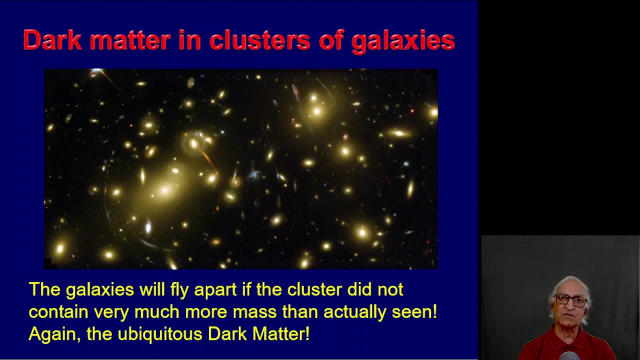 was non-luminous, but it nevertheless exerted gravitational influence, And this matter has come to be known as dark matter. Dark matter exists not just in individual galaxies, but also in clusters of galaxies. That was conjectured way back in the 1930s by the Caltech astronomer Fritz Zwicky. 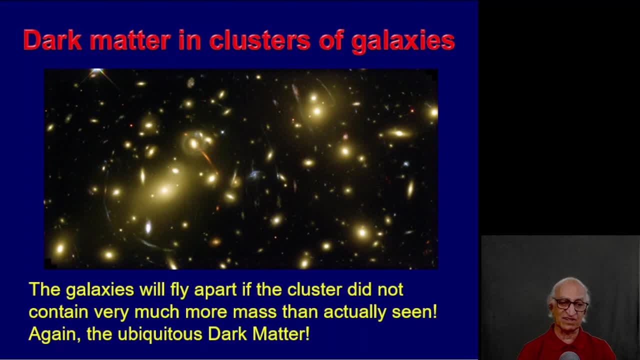 Zwicky argued at that time- and nobody was willing to take him seriously- that they could create a galaxy in a cluster that would fly apart if the cluster did not have very much more mass than can be accounted for by the luminous galaxies themselves. 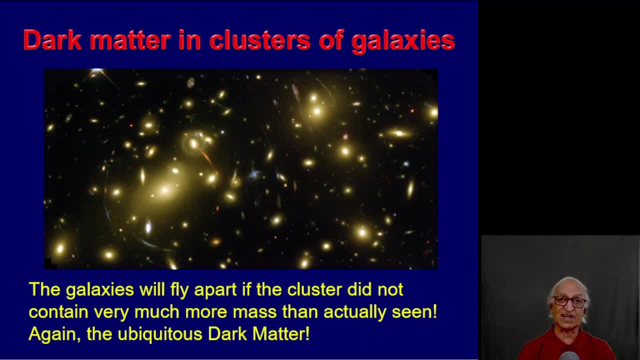 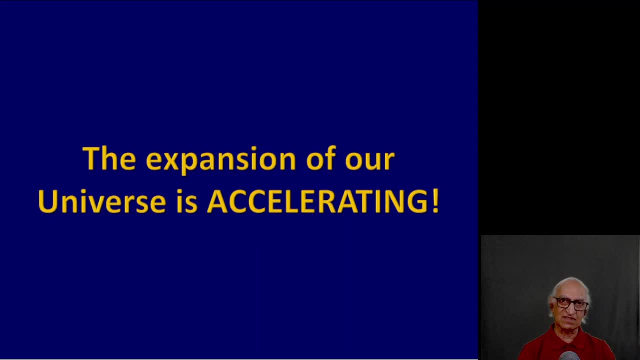 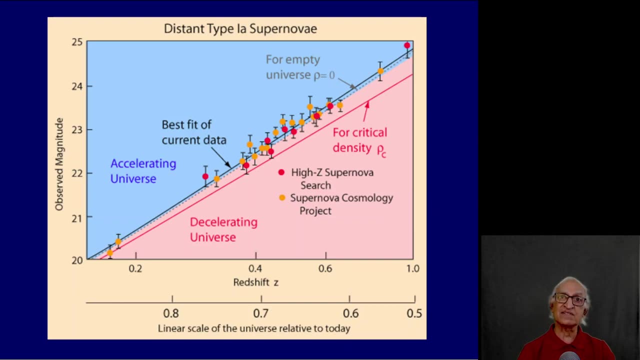 He conjectured that 90% of the mass of the clusters of galaxies must also be this mysterious dark matter. Around the year 2000,. astronomers made a startling discovery: that the universe is not only expanding, but expanding. The expansion is accelerating. 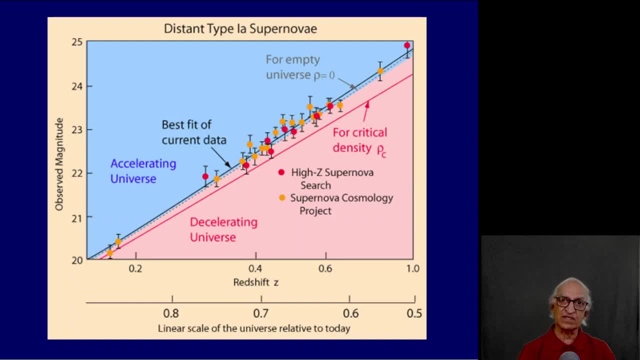 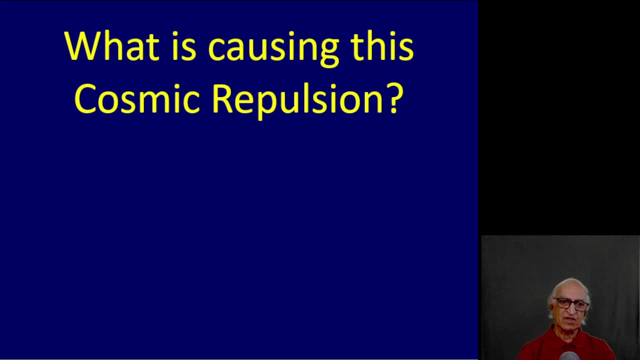 What one would normally expect is that the expansion should be slowing down, because the gravity will pull the matter back to the universe. If the universe is in fact accelerating its expansion, then something must be pushing it. Physicists have termed this mysterious source of cosmic repulsion as dark matter. 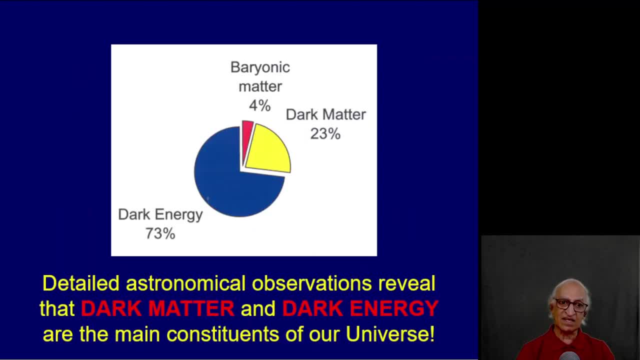 The dark matter is the dark matter that is the basis for the dark energy. Observations clearly now demonstrate that normal matter, such as matter that we are made of and we are familiar with, constitutes only 4% of all the energy density of the universe. 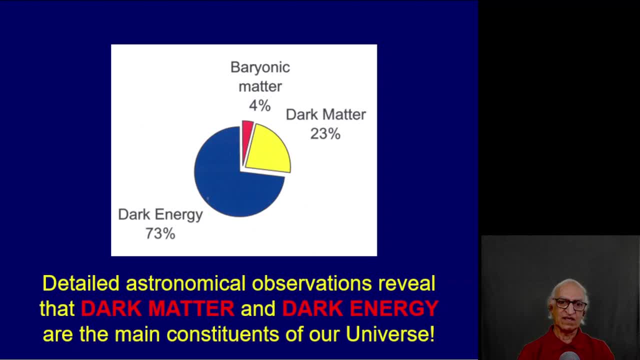 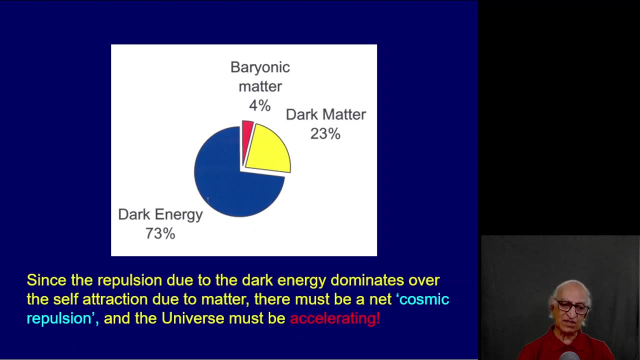 The remaining 95% or so is rather mysterious. There is this dark matter which constitutes 23%. But dark matter is also mysterious. It's a dark matter which is capable of transforming itself. It's a dark matter. matter provides attractive gravity, but the dark energy, which is 73%, provides repulsive. 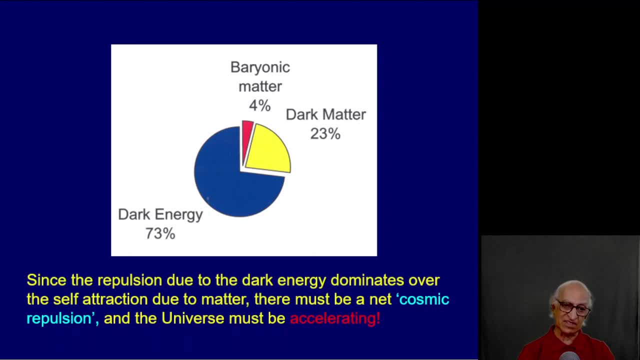 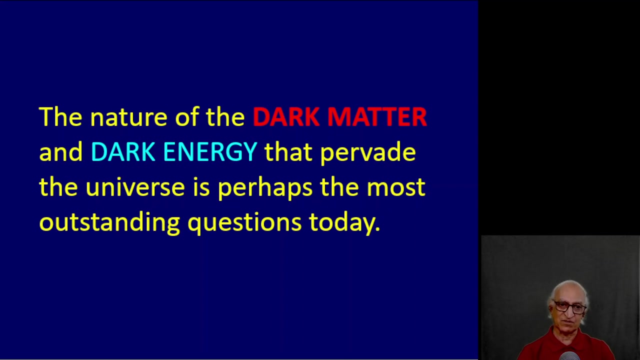 gravity, And since dark energy is 73% and matter that provides attractive gravity is only about 27%, the cosmic repulsion wins out, and that is why the expansion of the universe is today accelerating. We don't know what this dark matter is at all. we don't know what this dark energy is. 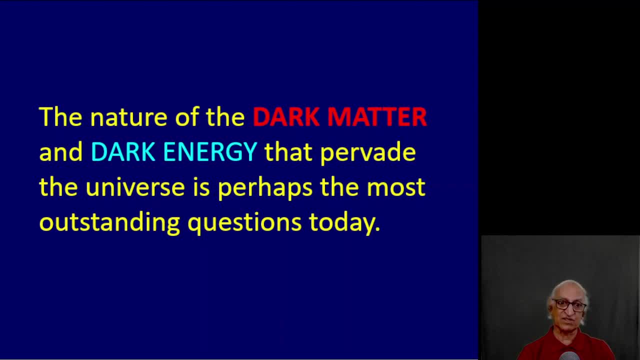 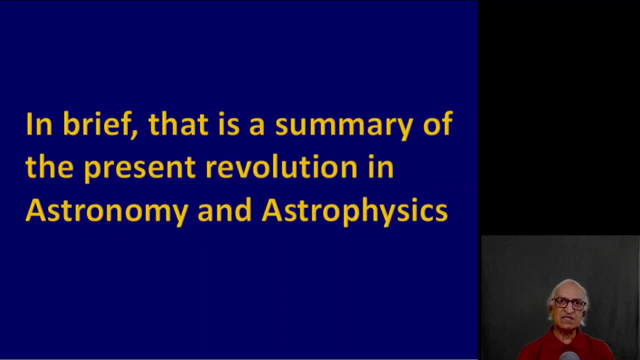 The nature of the dark matter and dark energy that pervades the universe is perhaps the most outstanding question of physics today. In brief, that is a summary of the present revolution in astronomy and astrophysics. Let us now return to the present. Thank you. 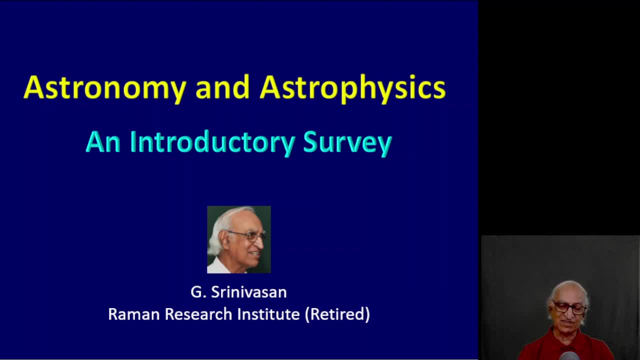 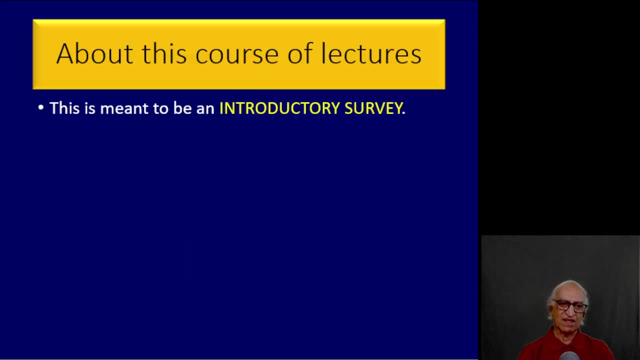 To this series of lectures of this, of which this was just the first lecture. Let me tell you something about these lectures. This is meant to be an introductory survey. I hope to cover all the topics that I mentioned in this overview in about 40 lectures roughly. 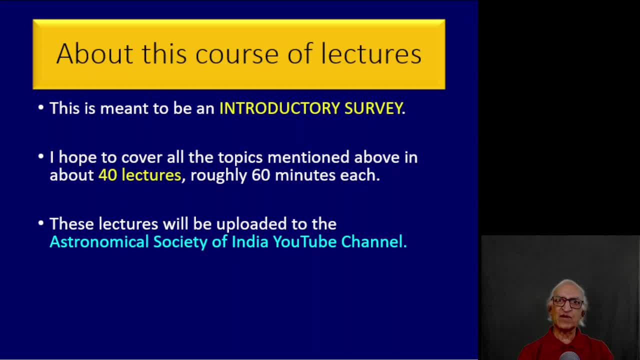 60 minutes each. These lectures will be uploaded to the Astrophysics Institute. You will find a link to the Astronomical Society of India YouTube channel. For further detail, refer to the website mentioned in the poster by the Astronomical Society of. 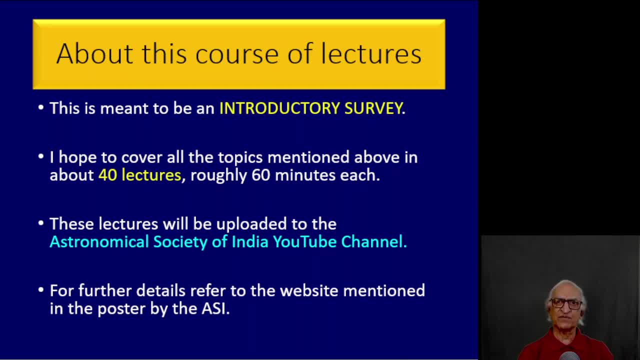 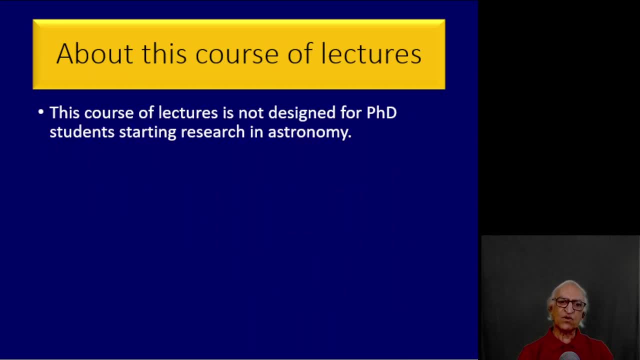 India, which was shown right in the beginning, And in any case, if you go to the website of the Astronomical Society of India, you will find where to go. This course of lectures is not intended for PhD students starting their research in astronomy. 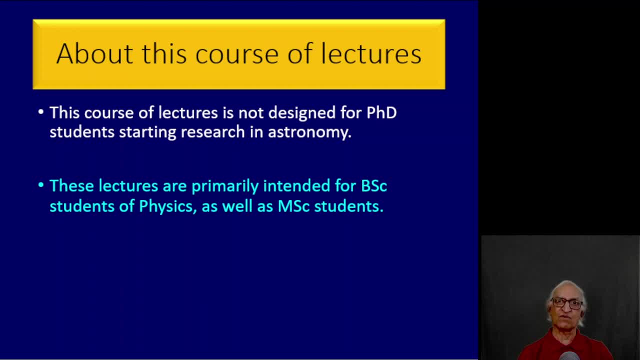 Okay, Rather, these lectures are primarily intended for college students studying BSc physics or MSc students. Engineering students may also find it interesting, and they will have the necessary background in physics and mathematics to follow these lectures. What do I expect you to know? 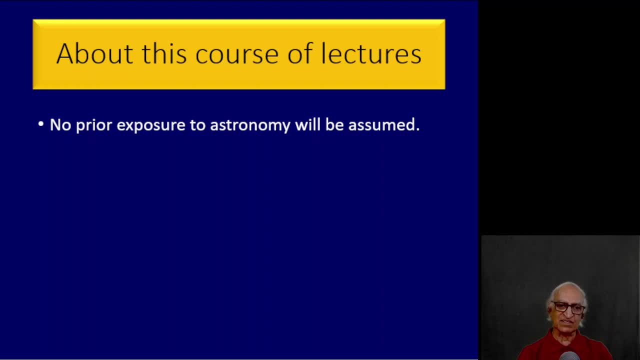 No prior exposure to astronomy will be assumed in these lectures. Research of physics at, say, Resnick-Halliday level of Sears and Zemansky University Physics will be required and should be adequate. Pre-university-level mathematics should be more than adequate. 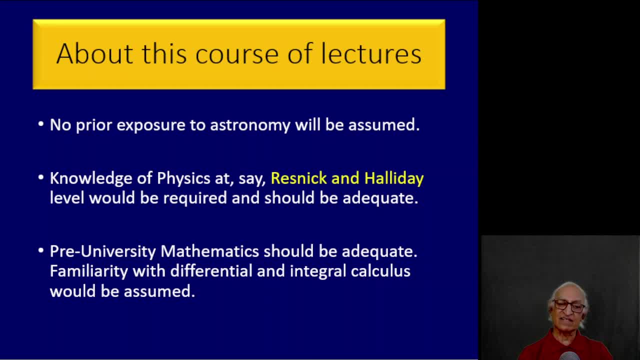 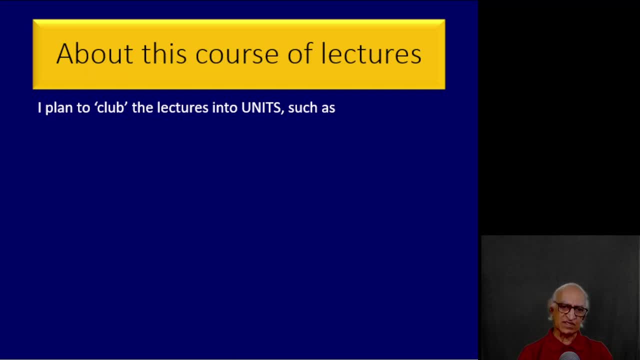 Some familiarity with differential and integral calculus would be assumed. I plan to club these lectures into units such as stars n, states of stars, White dwarfs, neutron stars, black holes, etc. The interstellar medium, galaxies, high-energy astrophysics, cosmology, etc.